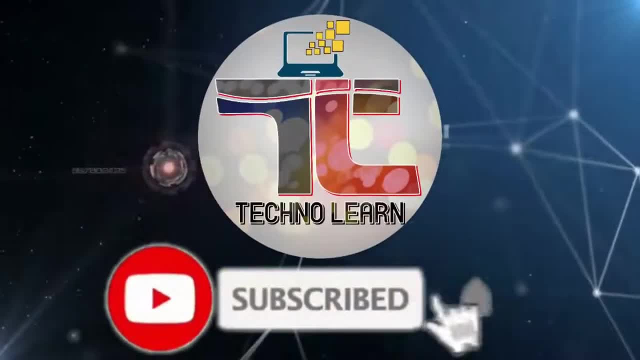 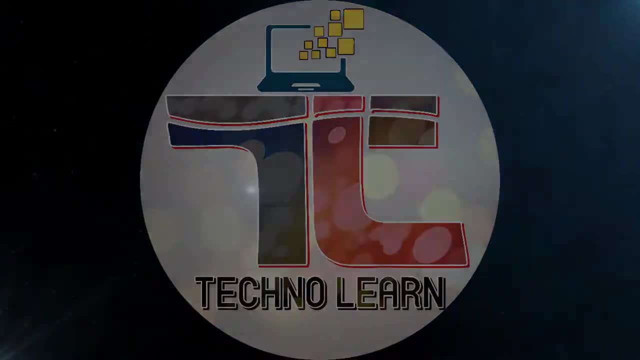 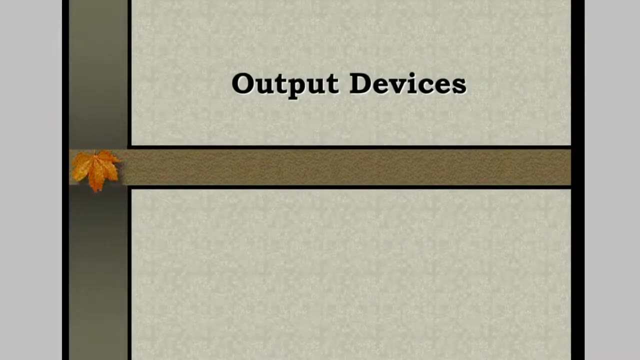 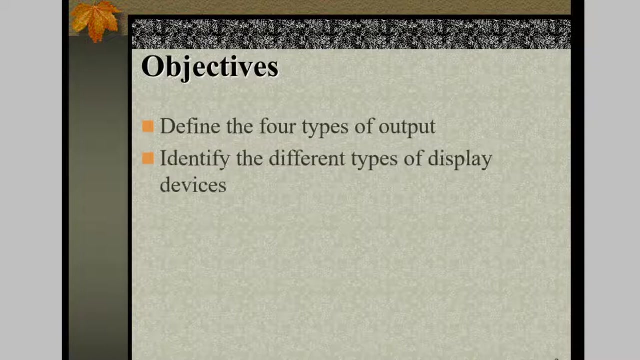 In this lecture we discuss about the output devices, types of output devices. what are the objectives of output devices? Our objective of this lecture is to define the four types of output, Identify the different types of display devices, Describe the factors that affect the quality of monitors, Understand the purpose of videos cards, Then identify. 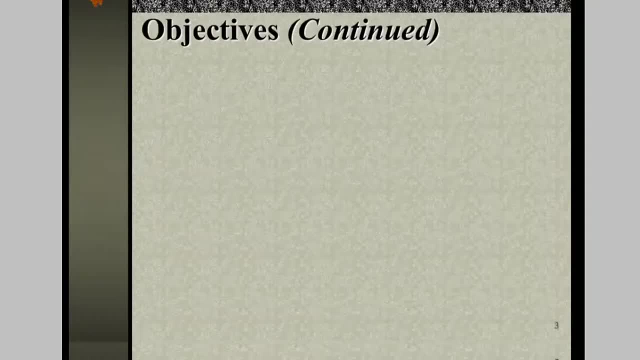 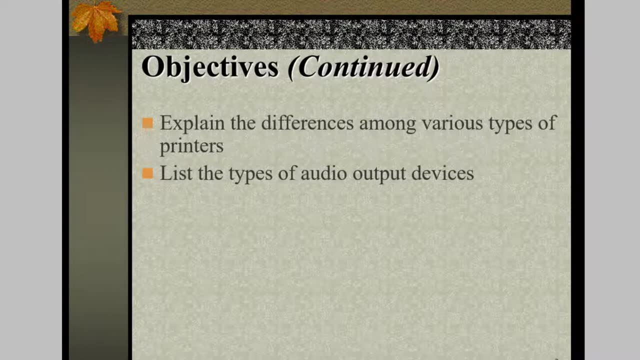 the monitor. ergonomics issues. Objectives: Explain the differences among the various types of printers. List the types of audio output devices. Identify the purpose of data projects. facts, machines and multifunctional devices. Explain how the terminal is both. 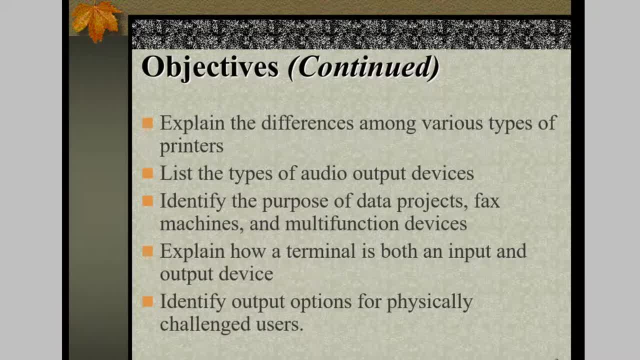 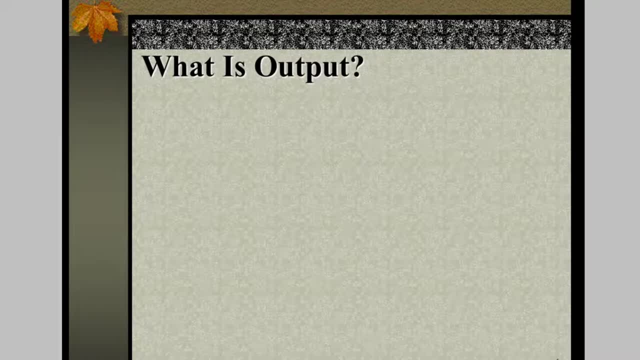 an input and output device. Identify output options for physically challenged users. What is output? Anything, computer-processed data and information and then, after processing the data and information, computer shows the result is known as output. There are different types of output. We discuss in this lecture about the four types text. 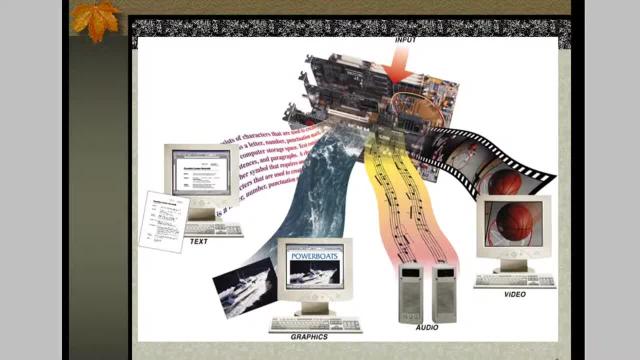 graphics, audio video. As you show in the diagram, there are different types of output we receive from the different devices. Computer sends the data or information to the user through the different devices. These devices are known as output devices. Output devices are the devices through which we receive. 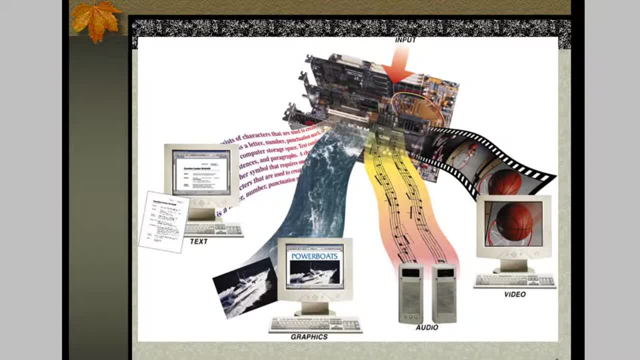 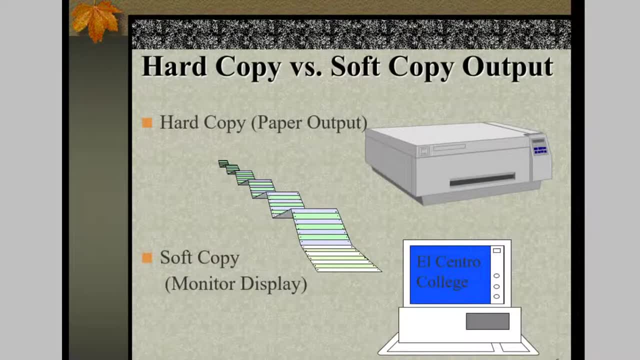 the data from the computer is known as output devices. There are different types of output. types of output: RS follows hardcopy and then softcopy. softcopy output, the electronic version of the document, is known as softcopy. you are a boss. electronic version. what I mean? K Joe Murray, computer again, the data store. 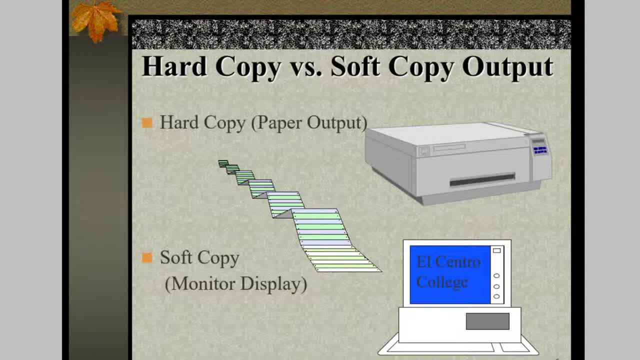 here is a device to a person over there in the form of files is known as soft copy output. a soft copy, the vacuum, while may your computer major data with a TK. basically, we're about to go to a soft copy of the electronic version. you would have a memory pass soft copy of the sitra jump printed version of the 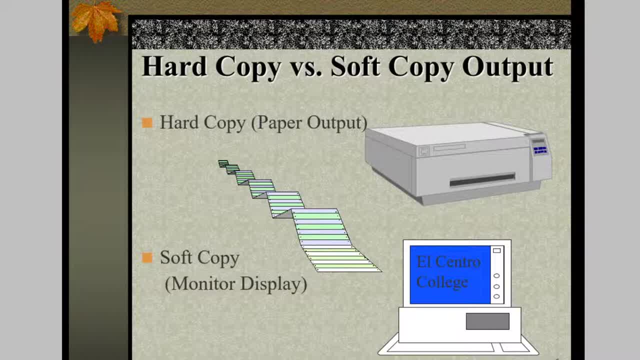 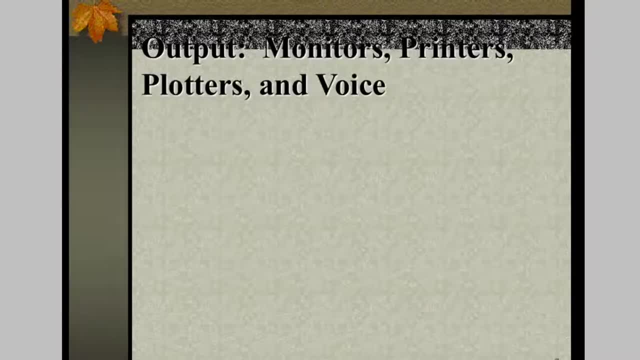 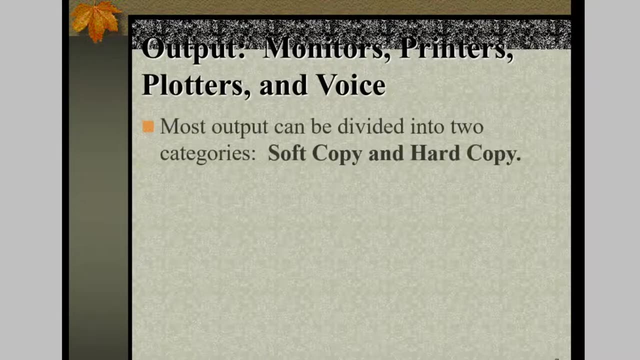 soft copy output to America. soft copy my data with a story of printed version with a the most complete. and so basically, Kevin, that I have a hard copy of my boss. output devices can- there I'm taking a- monitors and printers and proctors and sitra wise, most output. 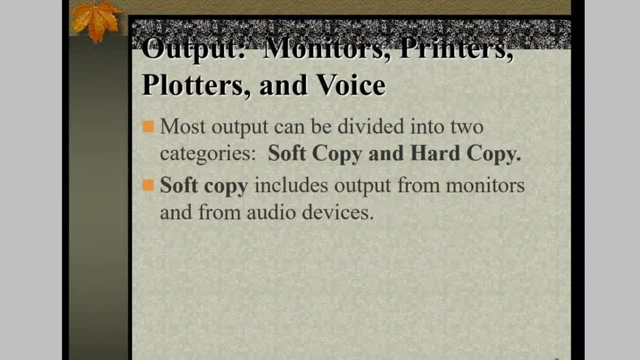 can be divided into two categories: soft copy and hard copy. so if copy include the output from monitors and from audio devices, just a very quick was produced. or yeah, yeah, my monitor stupid. or data, sure, I just say we have local. put in another area to you, my boss. soft copy, a hard copy. 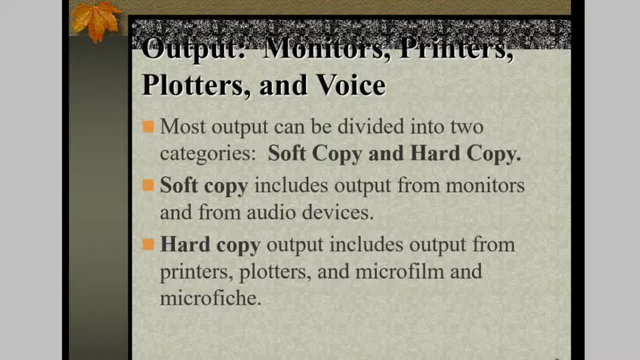 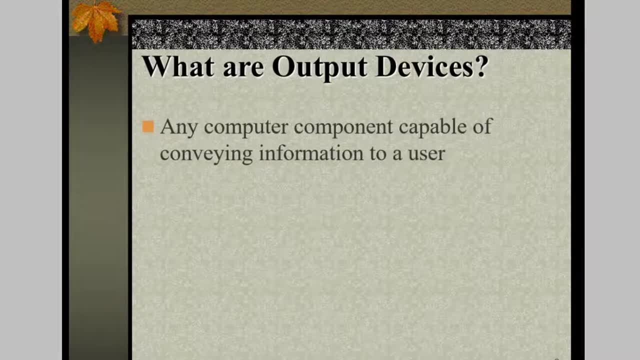 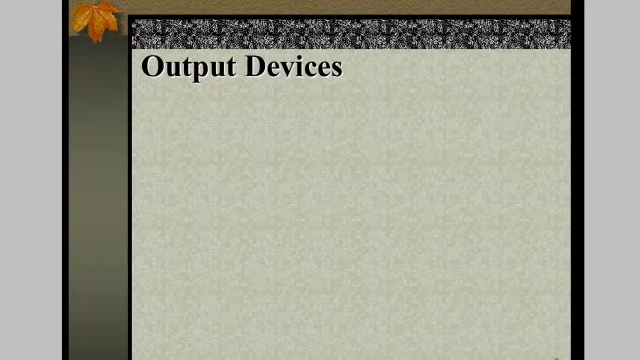 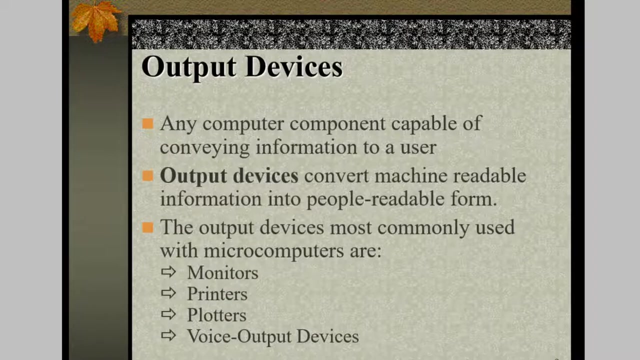 output is that? so that was a super high level roll footage of the enfermed Europe machine-readable information into people anybody won't form. yes, are you have a very, very great of socket인이 under the spizza? I think the Chinese power supply literally a 00 file generate. was paper model broken? the other I have you got to bibitım. 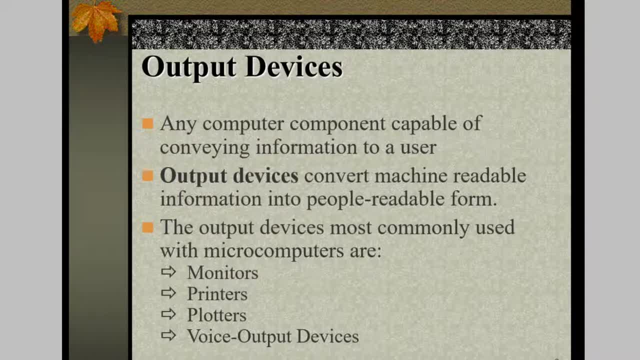 It was also mentioned in the previous input devices that when we start entering our information into the computer, the input devices first convert it into such a form that the computer can process or store. Similarly, when we talk about output devices, when we have data, the save in the computer first plays the role of the output device, then the output devices convert it to be human, readable or understandable for the user. 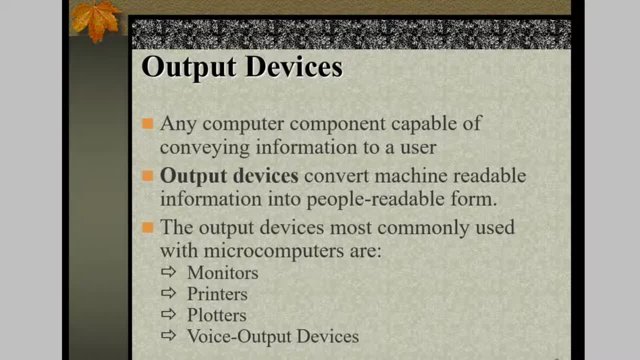 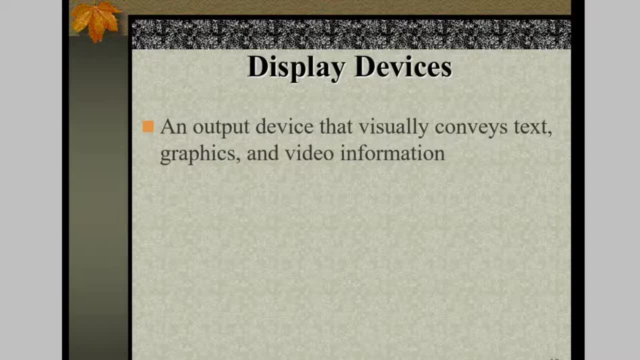 The output devices most commonly used with the macro computers are monitors, printers, plotters and voice output devices. Any output device that visually conveys the text, graphics and video information is called a display device, For example CRT monitors, cathode rays, tube monitors, screen housed in plastic or metal case, color monitors and monochrome monitors. 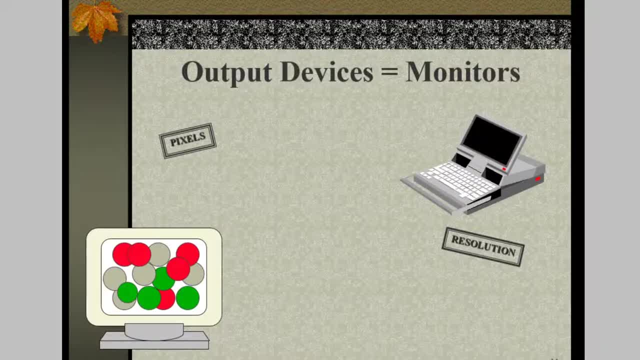 For example, we have these two types of monitors: In the form of pixels. we have output devices. Output devices are monitors As we have. it has a resolution and pixels. So today you will also understand what the resolution is, what the pixels are. 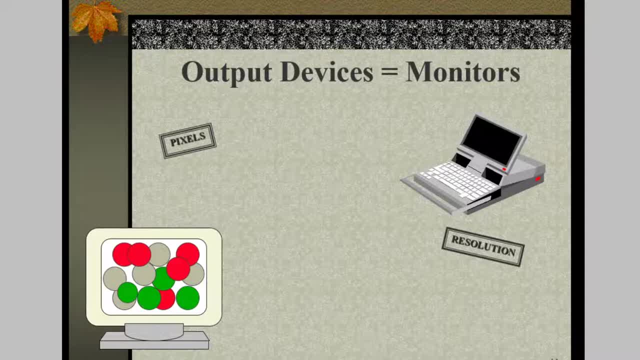 And when we talk about our camera, whether it is 4 megapixel or 8 megapixel, then we also talk about the quality of the 8 megapixel one. The quality of the 4 megapixel one will not be good, So we don't know why. 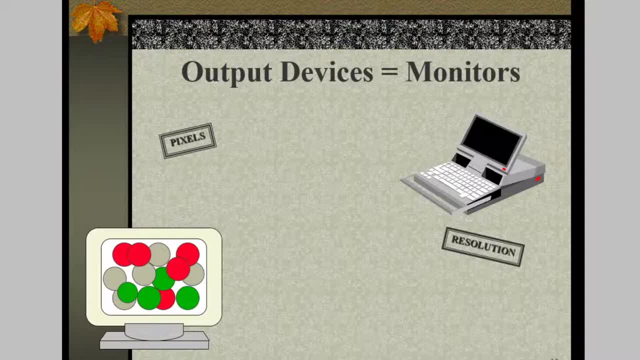 So today we also have to see why its quality is so good and what is the resolution. We have different types of monitors. We have CRT monitors, As you can see in the diagram here. I highlight it with a highlighter. You can see the diagram we have. 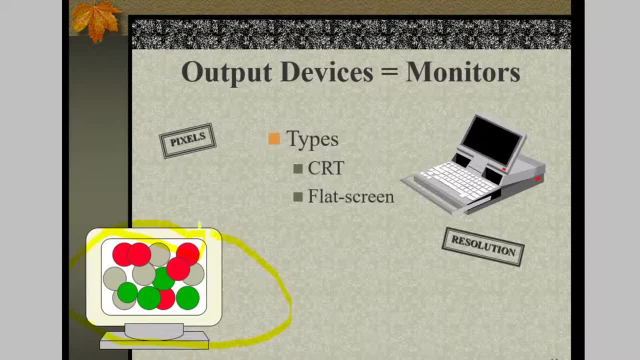 We have CRT monitors like this. We have flatbed monitors like this. We have simple screens like LCDs. So we have flatbed monitors. So these are the types. What is its resolution? We have to discuss that further. Its resolution is that how many pixels we have, or how many screens it will use to display. 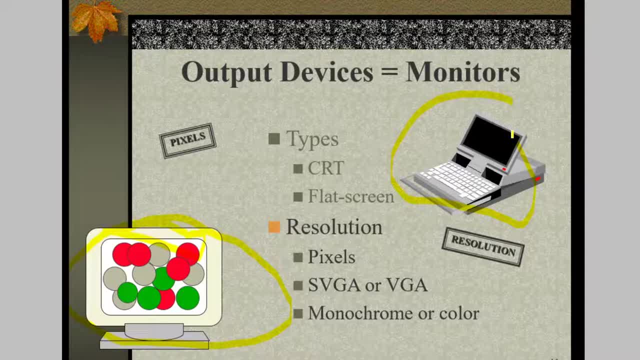 It is called its resolution. We will see about pixels. We will discuss about SVJ and VJ videographic adapters. We will discuss the super videographic adapter that we will have. We will discuss monochrome and color. We will discuss all these things further. 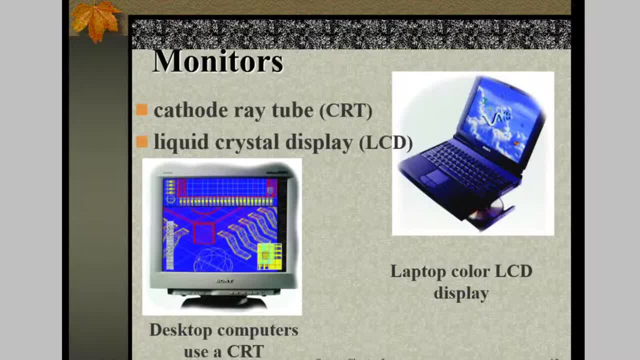 Now here we have the monitors. We have cathode ray tube, CRT, liquid crystal display, LCDs. We have desktop computers. We used to have CRT monitors, But now you will see that mostly we have LCDs. Most of the laptops used to have LCDs. 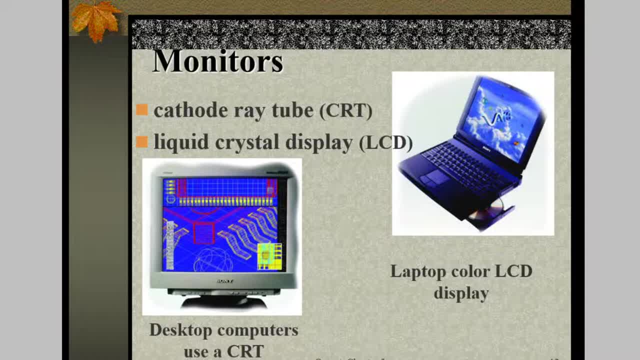 But now we have desktop computers. They also use LCDs. So we have a cathode ray tube in the CRT monitor. You must have heard of it. Earlier television used to have a picture tube in it. Now we are not going into the details of how it works. 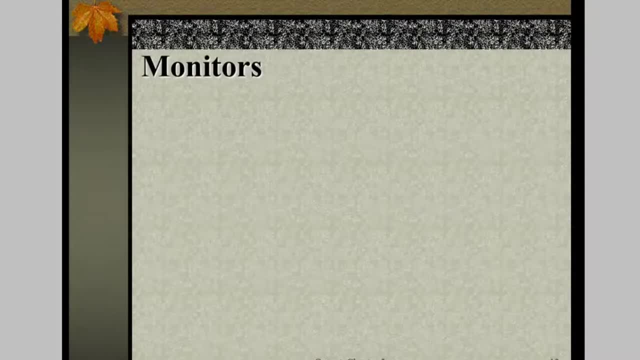 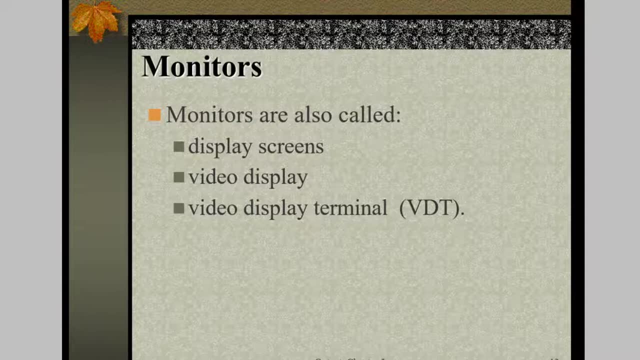 Just for your information that what are these output devices? So we have monitors. Monitor is also called display screen. It is also called video display. Video display terminal is also called VDT, Which we have monitors. Similarly, if we talk about the monitors, 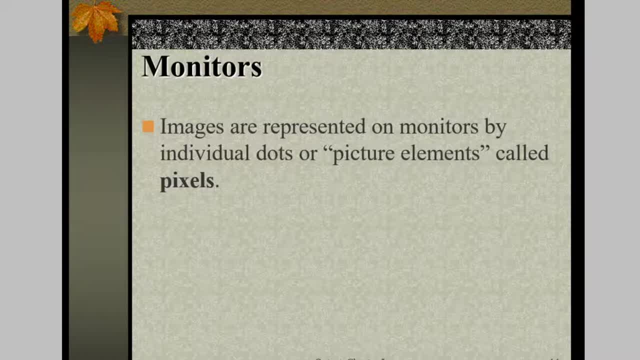 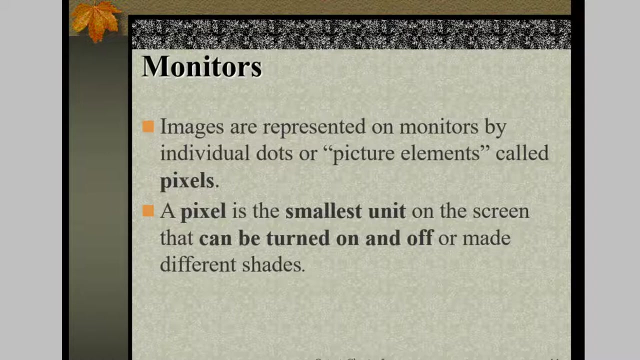 Images are represented on the monitors by individual dots. The images on the screen are represented by dots. The dot is called picture element or pixel. Because the picture is represented by dots, It is also called picture element or pixel. A pixel is the smallest unit on the screen. 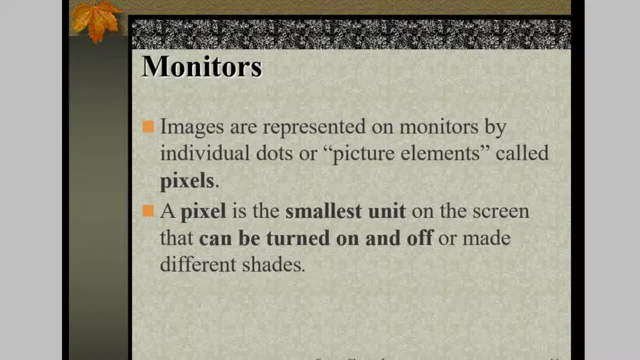 That can be turned on and off on the main screen, Like what will happen on the screen Will be on or off, In different shades, In different shades In different colors, Which you see Like here you are looking at the diagram. 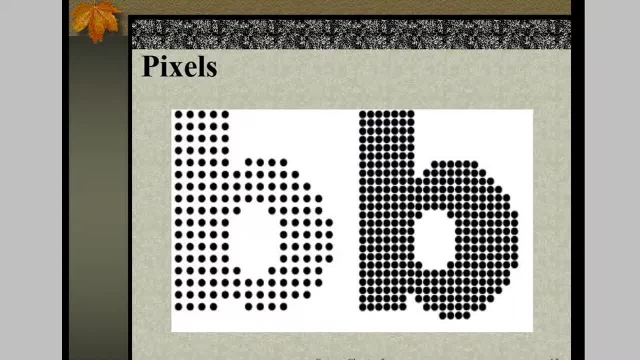 What do we have here? This is B. What else do we have Now see, which one do you see more visible? First one, This one you see more visible. Or this one you see more visible? I see this one more visible. 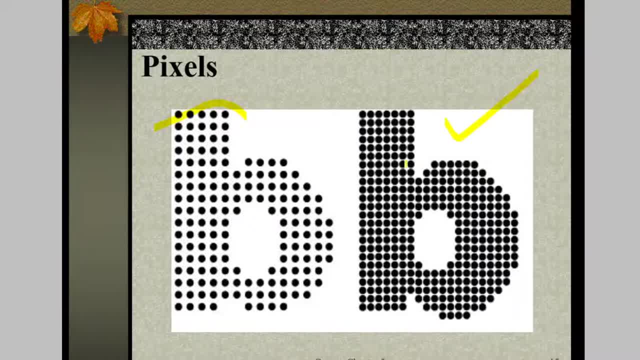 What is the reason for that? Because its dots are more. It has more pixels. It has more pixels. If its pixels are more, Then it will be close. Then what will be? the same picture. It will be clear When you make a picture with your camera. 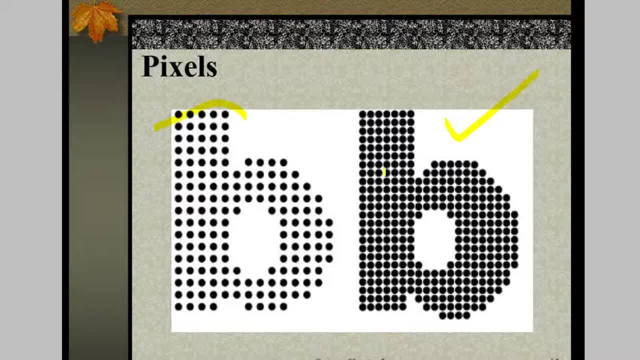 Whose pixels are more. Then you see the weight And whose pixels will be less Like. if we have 4 megapixels, Then its low quality. If we have 8 megapixels, It means that it is using 8000 dots. 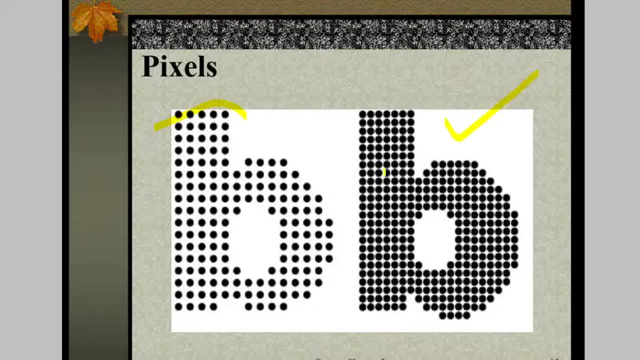 At least To make a diagram for you. So the closer they are, That's what we see. The picture is visible, Okay, And the thing is, When you zoom it, What happens? by zooming, It gets far away. Our pixels are getting far away. 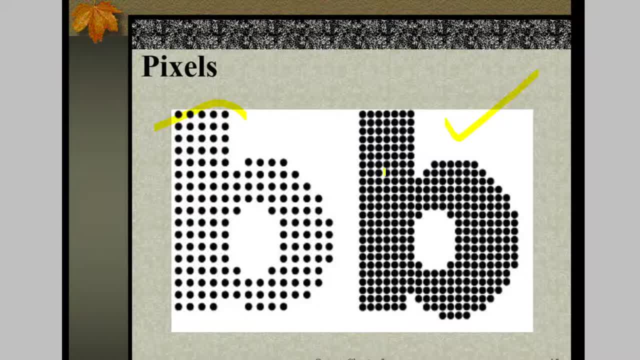 So the one whose pixels are less. It quickly seems to us that it is bursting. Okay, Like we have. Whose pixels are more We zoom it, more We see the words. So pixel means That all my pictures are made of dots. 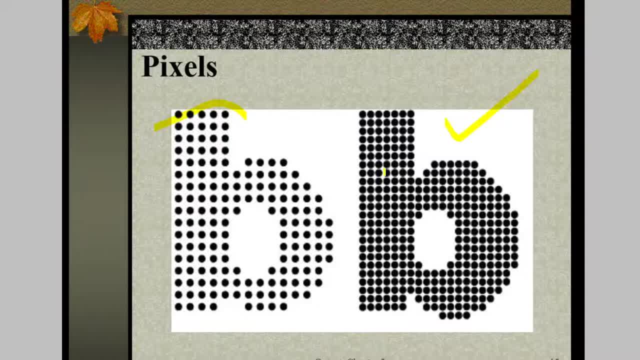 Whenever you make pictures in the camera, Then it is made of dots. We have a picture element, Or what will we call it Pixel? We will call it pixel. So wherever the pixel has to be highlighted, It turns on. The rest are called pixels. 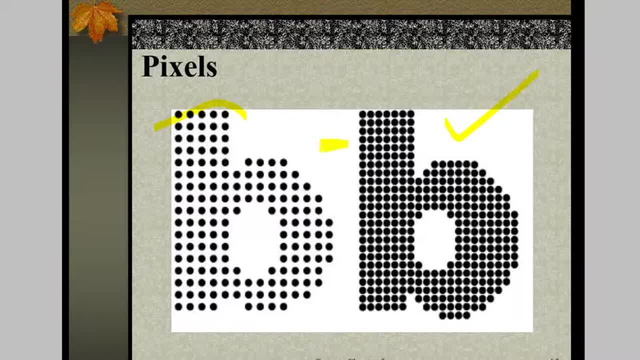 Here you can see this white place Now. it doesn't mean that there are no pixels on the screen. The pixels are present, Okay, The dots are present, But what are the dots we have? They are not active. Okay, This time they will not be highlighted. 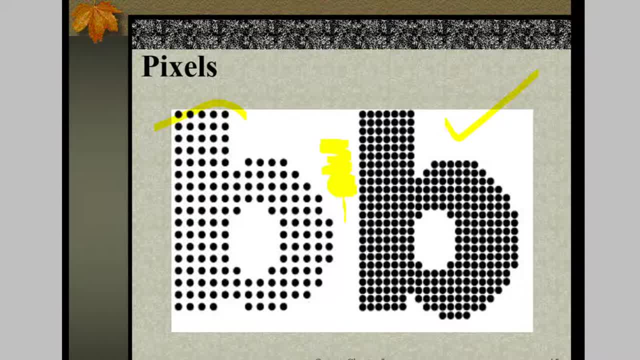 They will not be on. They will be off In the same way When you talk about the video. So what is the video we have? There are still pictures in it. Okay, Video is not that We have direct. We say that this video is being made. 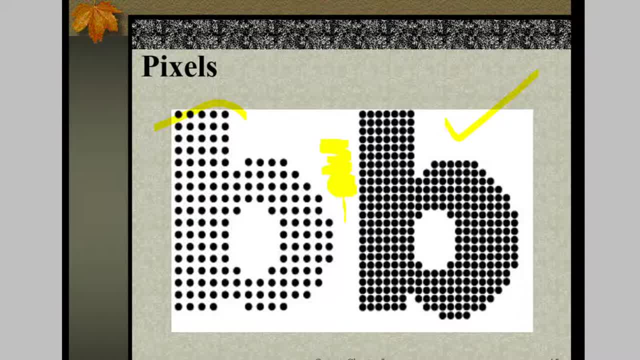 Pictures are also being made in it, Which we are making a video with our camera, So pictures are also being made in it. Pictures are being made, But they are being made in such a way Like in it. Frames mean that Forty-eight frames. 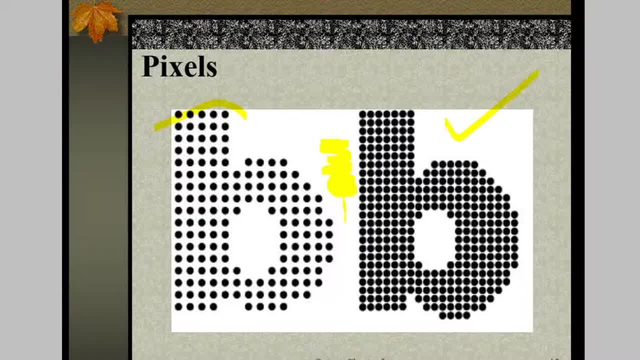 Or thirty frames. It means that In one second So many pictures have to be taken And then they have to move in one second. So we feel that, Like our what is happening? Video is happening, Movement is happening, What happens. 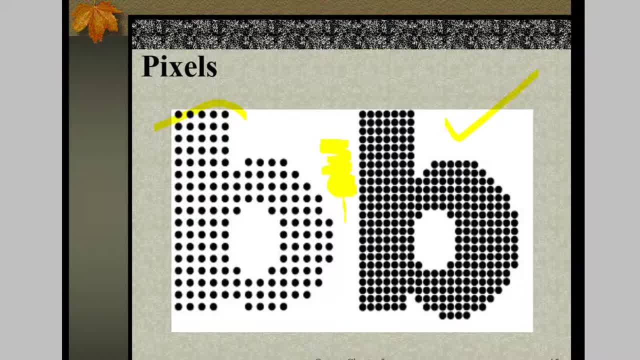 They are also pictures. Pictures are only Okay. What are our pictures? They are moving quickly. They are moving quickly, So we feel that Video. Now, when you put your hand up or down Or like this, I am making a video. 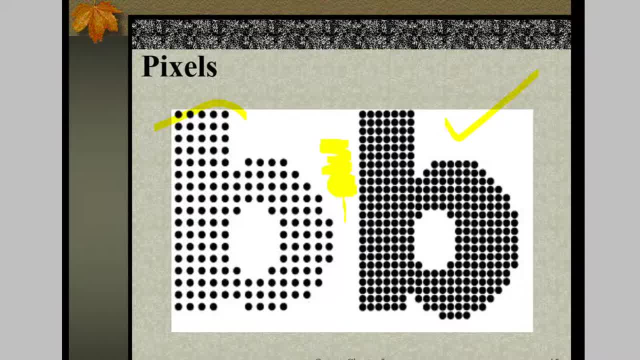 And in one second If he takes thirty pictures. So you see your hand A little bit, Wherever it will be. So many pictures are being taken So you will see your whole hand Moving. So in the same way We have a monitor. 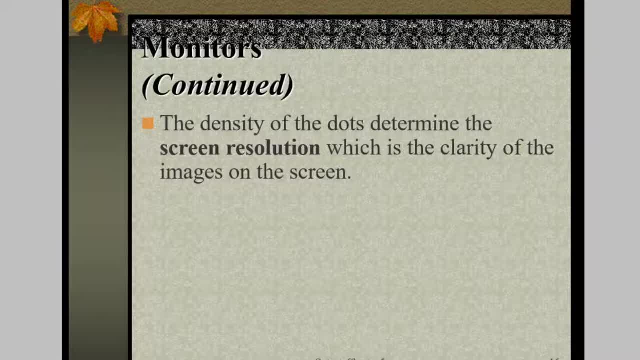 The density of the dots Determine the screen resolution. Means How many dots Dots are being used, How deep We have. That tells us the screen resolution, Which is the clarity Of the image on the screen. Because of this, 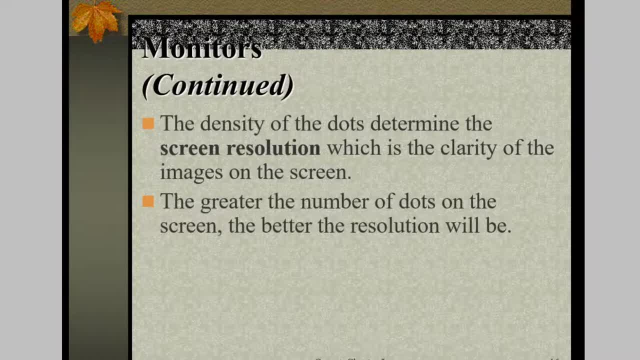 We have On the screen Clarity. The greater the number of dots On the screen, The better the resolution Will be. As much as we have, The more pixels They will be, So dense I mean They will be close. 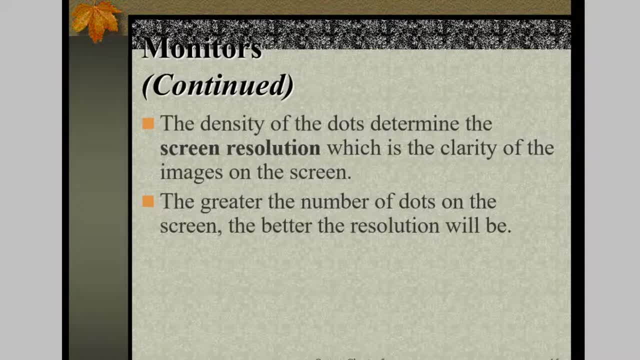 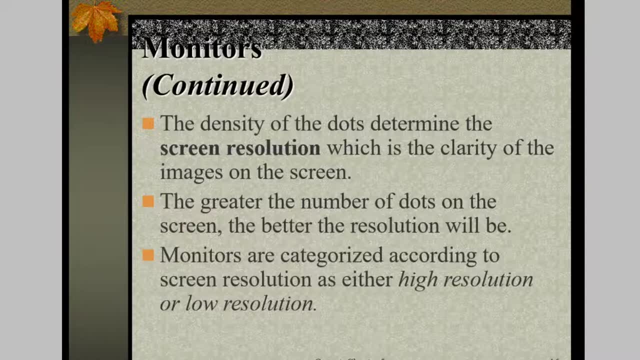 Close. Okay, As close as they are, As close as they are, So that What will be the clarity Will be More So. the monitor are categorized According to the screen resolution As either High resolution Or low resolution. 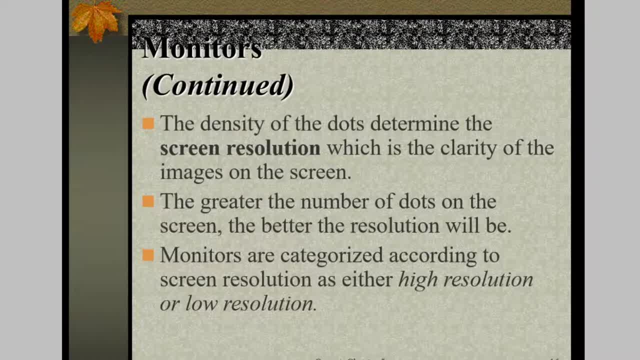 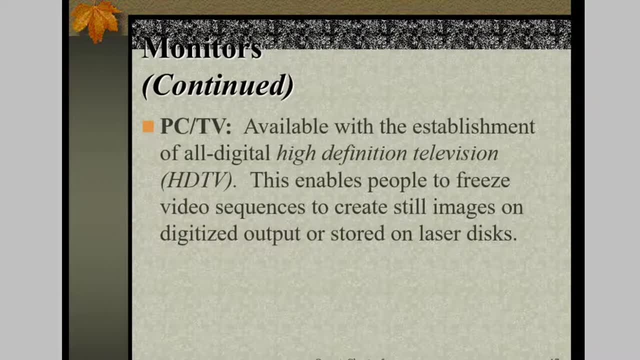 We have. You must ask How much does its resolution Support When the monitor goes to take our LCD? So we have High resolution. We have Similarly PC Or TV When you see, Available With the Establishment. 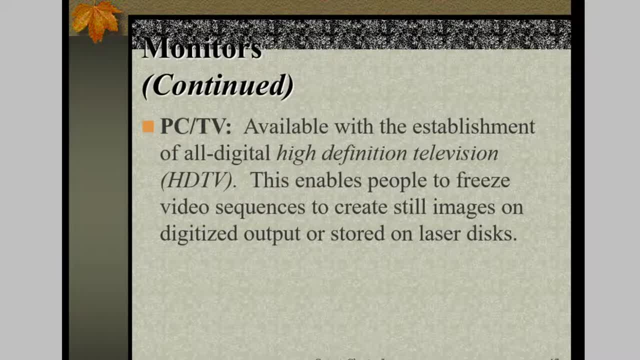 Of all digits. Digital High Definition Television, HDTV. When you hear this name, What is HDTV? Digital High Definition Television- Okay, This Enable The pupil To freeze Video Sequences. 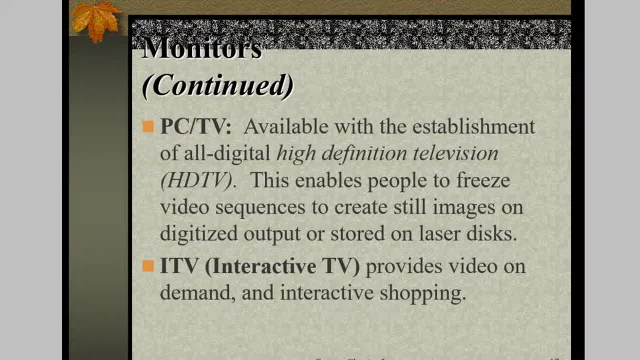 To create Still Image Teens. What is This Does not mean That This Is What This Is. This Is the Parameter In which The size Of Of the TV, The 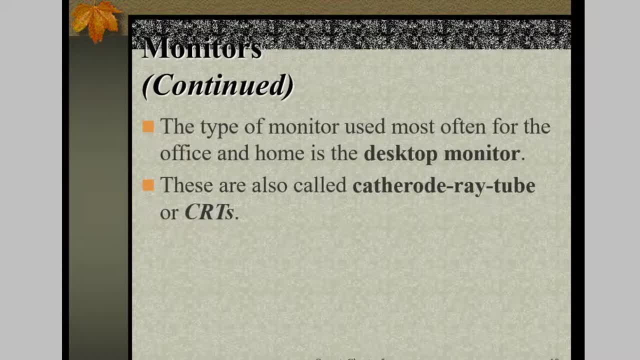 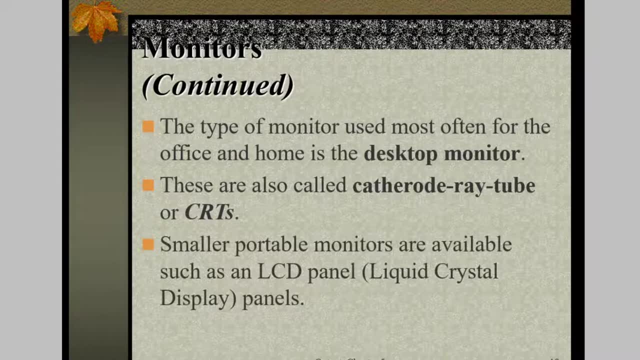 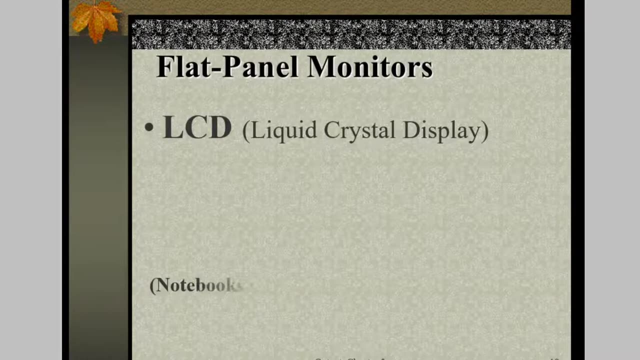 In which- There It is- 2., 2., 1., 2. The 3. 2.. Smaller portable monitors are available, such as LCDs. We use them a lot. Where do we use LCDs? 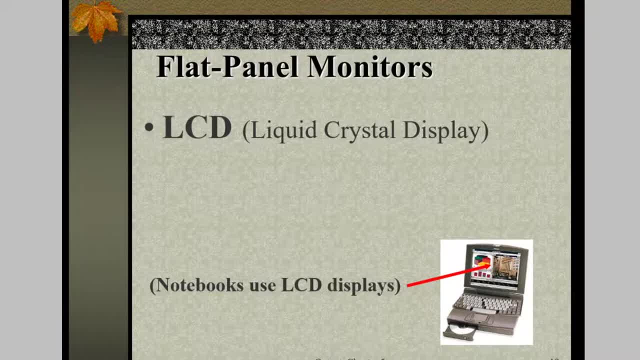 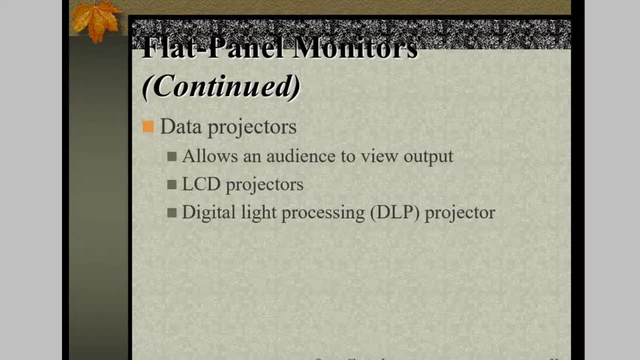 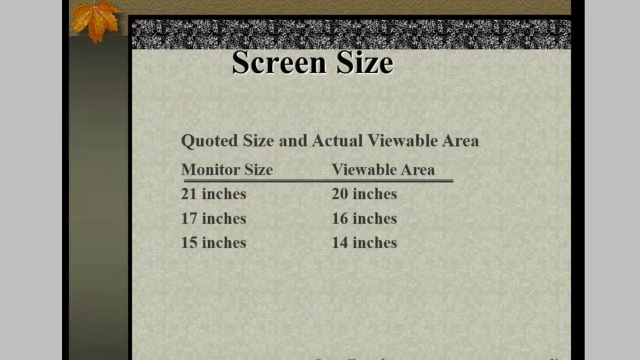 Notebook LCD display. We use LCDs for laptops, But mostly we use LCDs for CRD monitors. We also have flat panel monitors. Data projectors allow an audience to view the output. LCD projectors, Digital highlight processing- DLP. 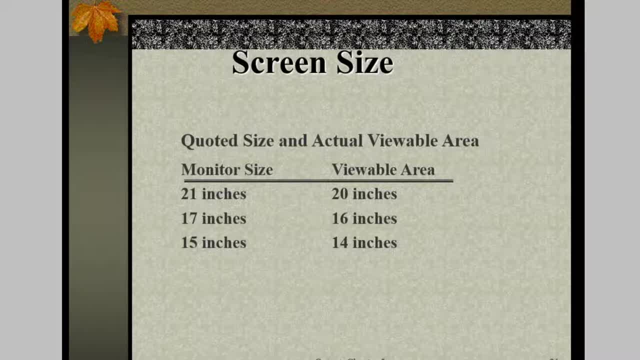 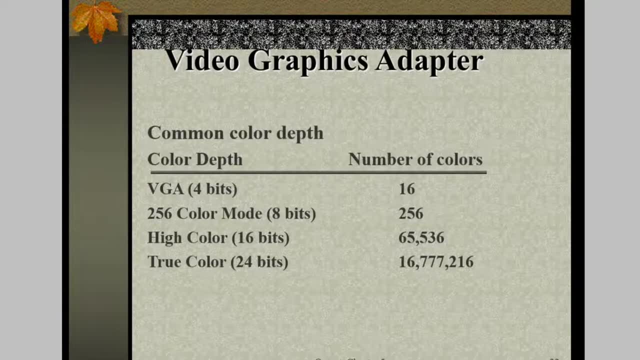 Screen sizes: 20 inches, 16 inches, 14 inches. Monitor size, Viewable area. Common color depth. Number of colors: 4 bit, 16 bit, 256 bit, 8 bit, 256 bit. High color. 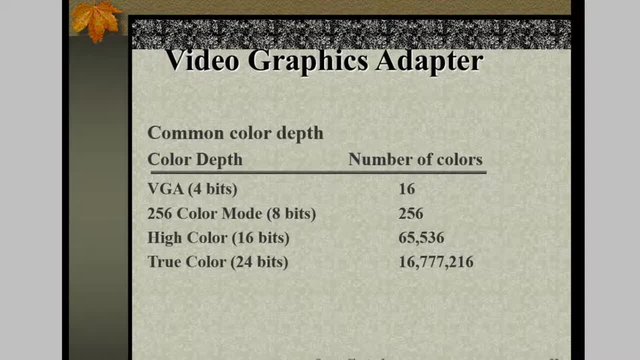 16 bit Color depth, 65530 bit Pro color. 24 bit Color depth, Common color depth. You can check it. You may have to buy these. You need to have such idea. We have resolution of the number of pixels. 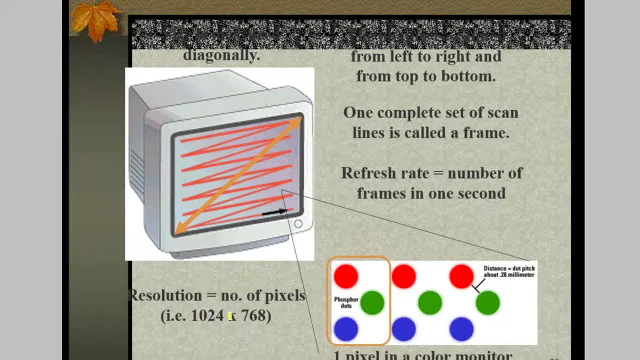 As per our instruction, when you are setting 1024x768 from left to right, you have to see this from top to bottom. once the complete set of scan lines is called a frame, so the complete lines are called frames. one pixel in a color monitor. so we have these dots. 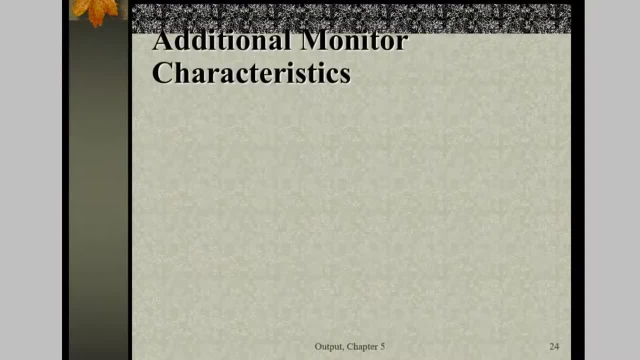 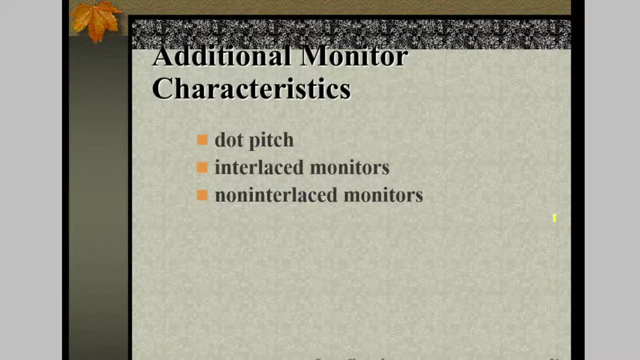 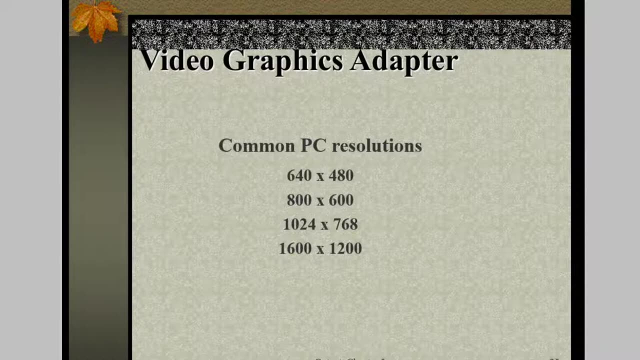 you are seeing, these are pixels in a color monitor. similarly, what are the additional monitor characteristics? dot pitch: we have interlaced monitors, non-interlaced monitors. we don't have to go into details, so these are the most used resolutions. when you are setting, 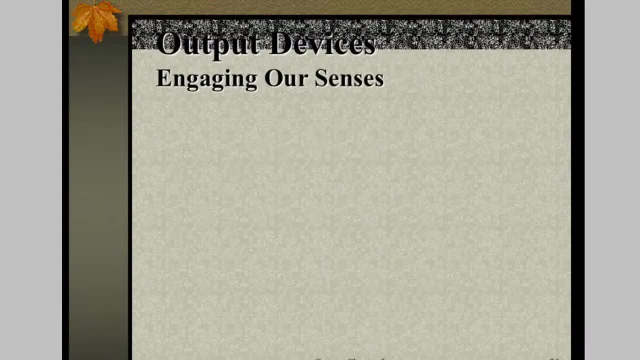 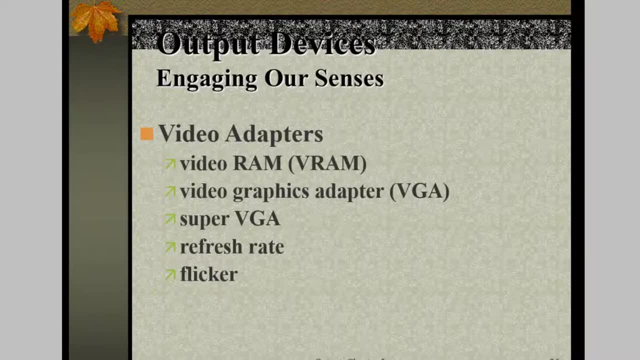 we have these resolutions, how do we set them? we will see later output devices engaging our scenes, like we have video adapters, video RAM, VRAM, video graphic adapter, VJ, super video graphic adapter, SVJ, refresh rate flicker. so these are different. 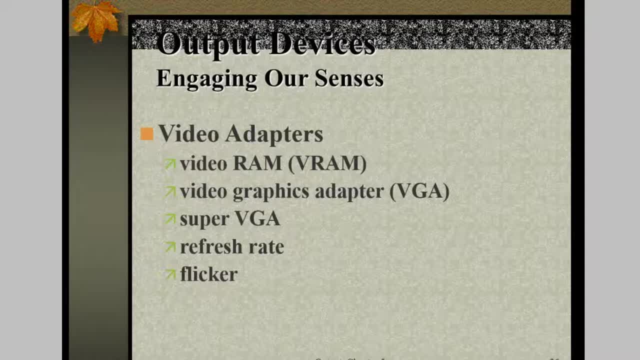 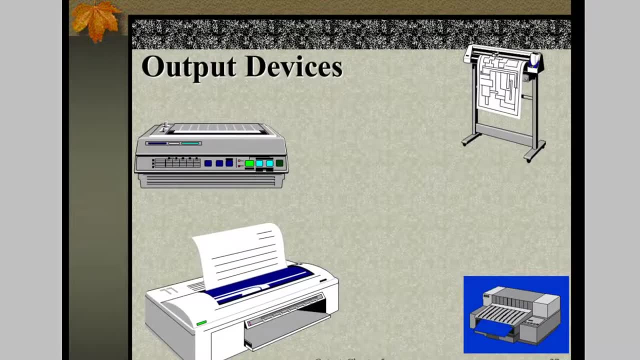 I am not going into details: what is VJ and what is SVJ, how we have SVJ quality as compared to the VJ output devices. these are different output devices. you are seeing like we have printer plotter. different types of printers are being used. flatbed plotters are being used. 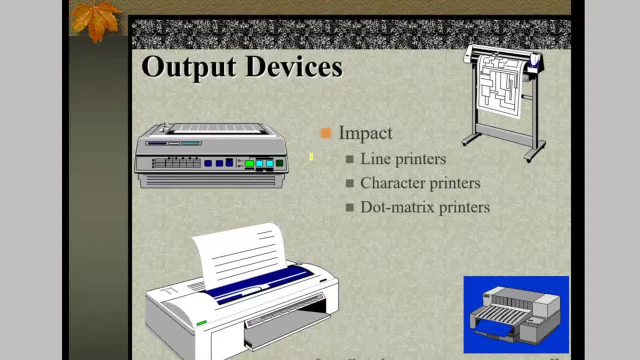 these are the examples of our output devices. now we have impact printer in which we have ink ribbon, or we have some component of printer which is touching our page. after touching, it is producing output. so these are called impact printers. like we have line printer, character printer, dot matrix printer, these are the impact printers. 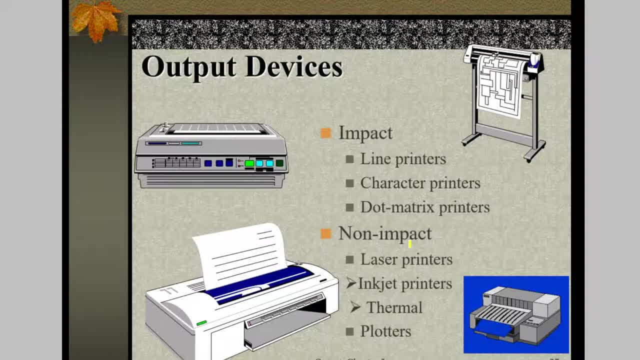 similarly, we have non-impact printers in which any thing, any component to print, to produce output, is not being touched. that is called non-impact printer. non-impact printer's noise is less. impact printer's noise is more and slow. non-impact printer's noise is less. 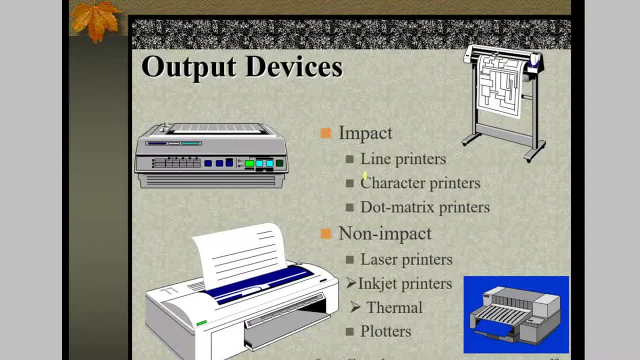 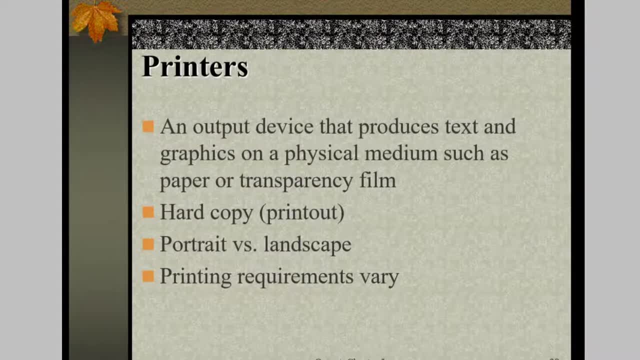 and their quality is also good. laser printer, inkjet printer, thermal plotters: these are non-impact printers. printers are the output devices that produce the text and graphics on a physical medium. physical medium means the medium which is present, like we have. 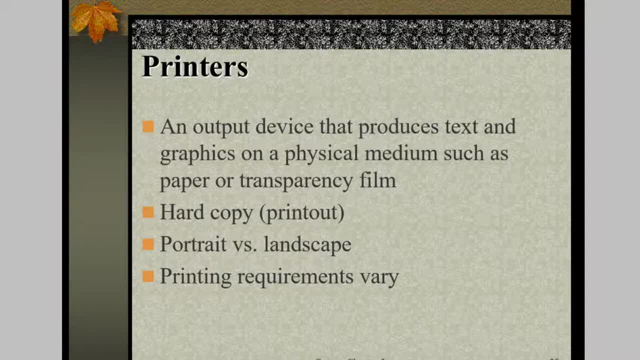 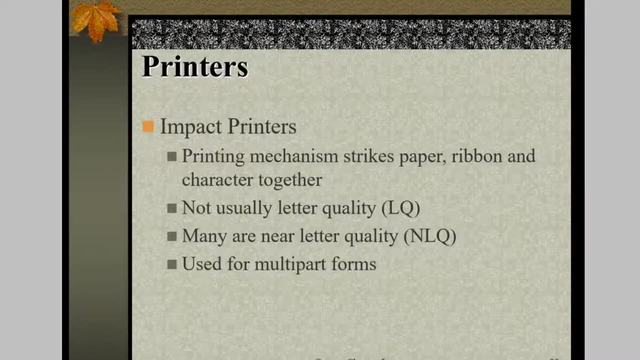 paper, such as paper, art, transparency film, hard copy printer produces print out similarly, portrait with landscape. we will see what is portrait and what is landscape. printing requirement vary now here: impact printer printing: the mechanism strikes the paper printing works in the same way, like i told you earlier. 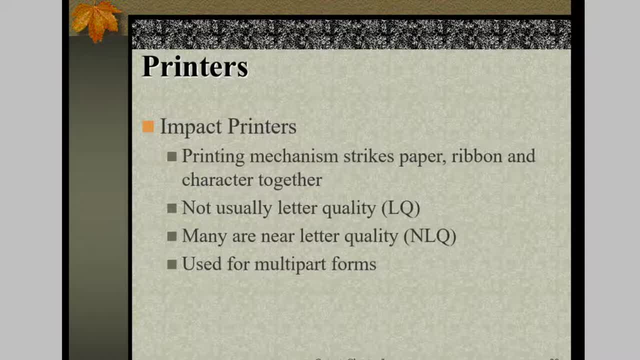 it will touch the paper with some kind of ribbon or touch with ribbon and then it will be corrected together. it strikes the paper ribbon and corrected together. they will be touching each other, not usually later quality LQ- similarly many are near later quality. 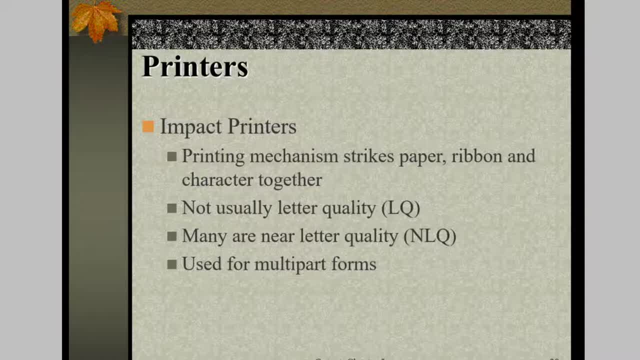 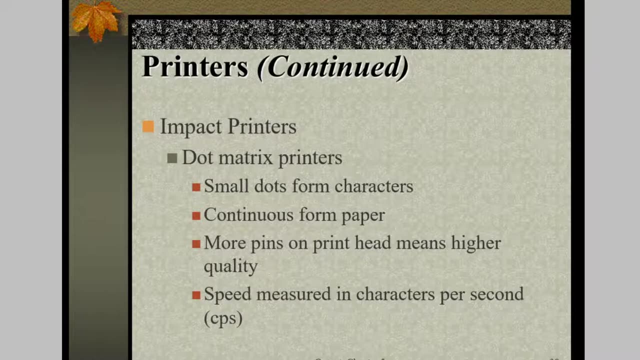 NLQ. we have now the quality we get. we do not have it now. earlier systems are used. now it is not used. use for multiple multi-part forms like. Next, we have Impact Printer, Dot Matrix Printer, Small Dot Form Corrector. Like when you used to go for shopping, they used to give you receipts. 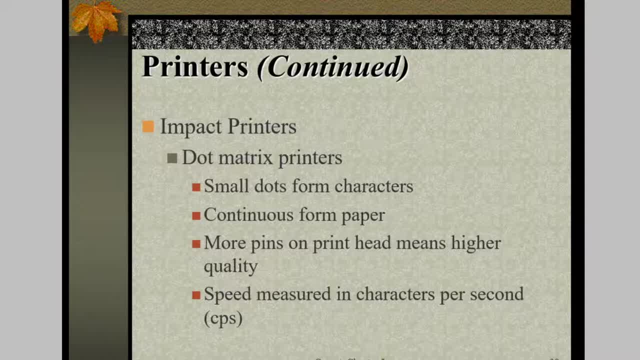 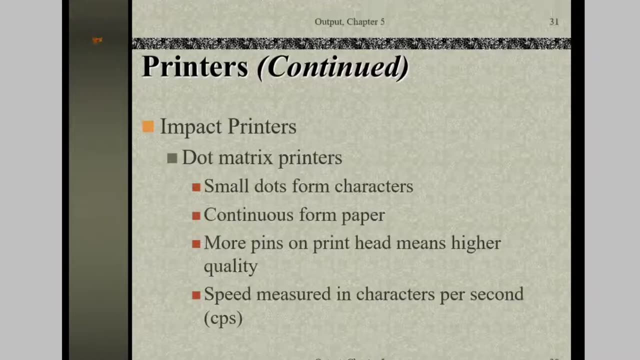 The output used to be in dotted form. Its quality is less and it costs less. More Pins: Continuous Form Paper. More Pins on the print. You don't have to go into details. It is measured in characters per second. It is measured in the speed of Dot Matrix Printer. 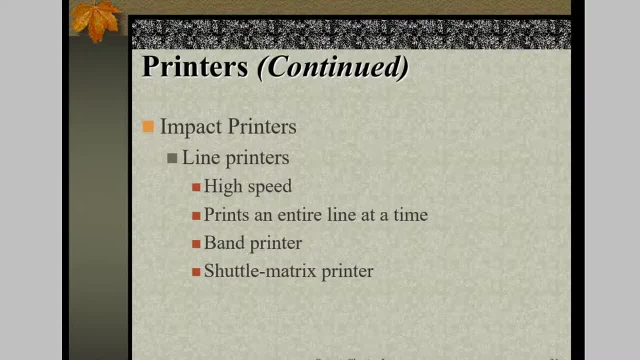 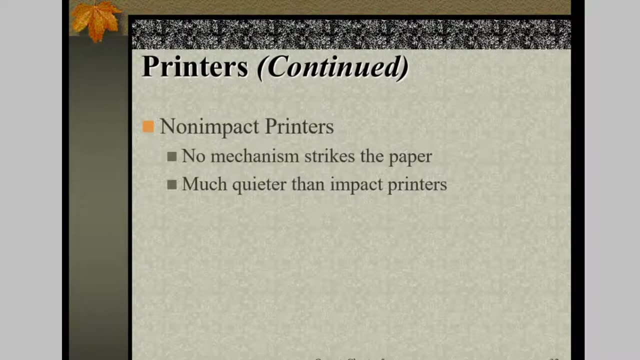 If we talk about Impact Printer, We have Line Printer. High Speed as compared to Dot Matrix Printer. It prints an entire line at a time. Band Printer, Shuttle Matrix Printer. Non Impact Printer: No mechanism strikes the paper, Nothing is touching the paper. Printing Mechanism- Much quicker than Impact Printer. 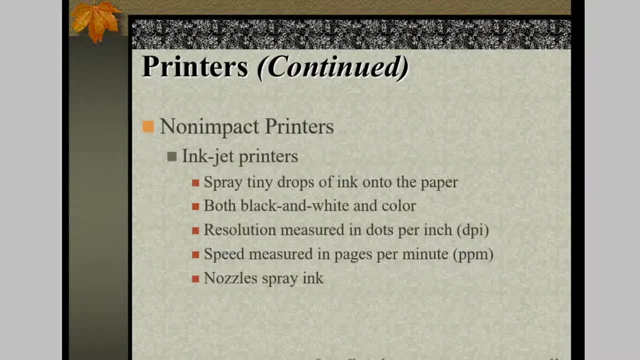 Impact Printer is faster than Impact Printer. For Non Impact Printer, we have Inkjet Printer. Inkjet Printer means ink spray. We don't spray like when you are polishing your shoes. Similarly, we have Ink Spray on the paper Spray tiny drops of ink onto the paper. Both black and white are available. 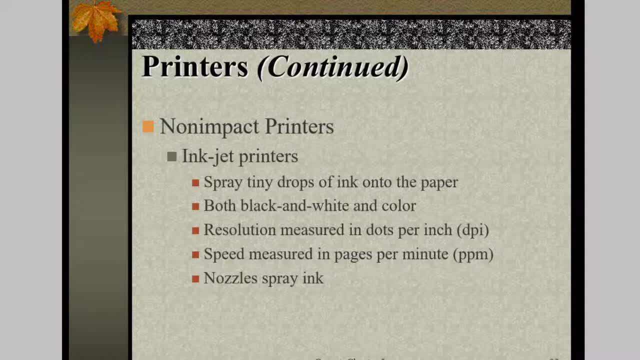 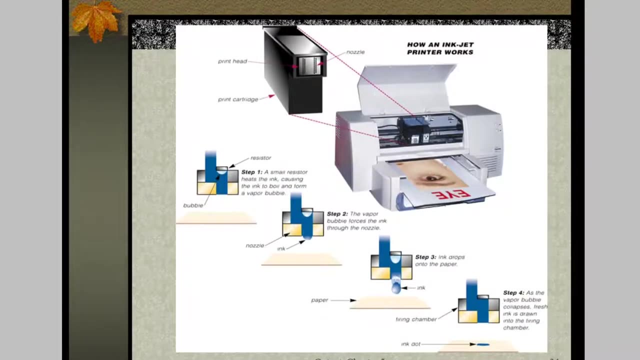 Inkjet Printer is black and white. Color Printer is also available. Resolution measured in dots per inch. DPI measured in 1 inch. Speed measured in pages per minute. How many pages will be printed in 1 minute? PPM Nozzle Spraying. I am giving you an overview so that these things are clear. 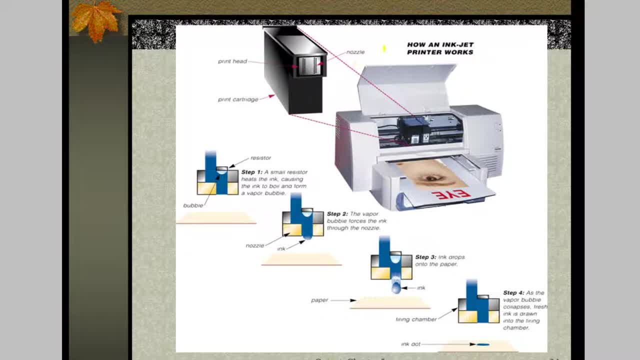 We have a print head. These are nozzles from where spray has to come. Inkjet Printer sprays. You can see how Inkjet Printer works. We don't need to explain in detail. This is the print head. This is the print cartridge. This is the cartridge. 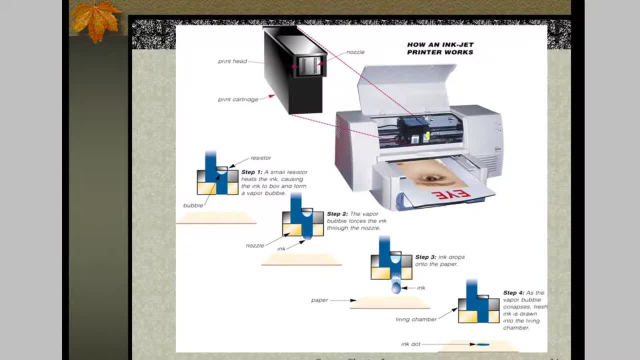 These are the nozzles. These are the nozzles. These are the nozzles. In the same way in step 1, Smaller Resistors. I don't need to explain in detail. It heats the ink. Resistor heats the ink, Causing the ink to boil. 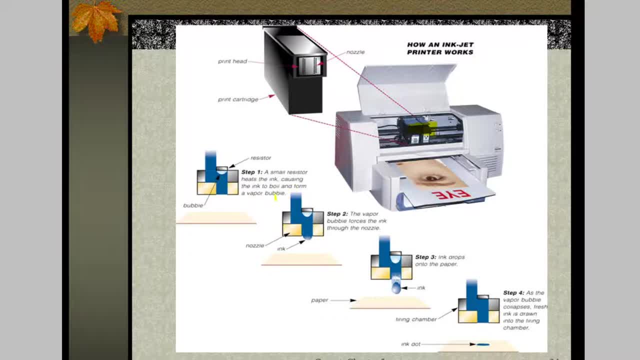 And forms a vapor bubble. The ink gets boiled and forms bubbles. In the same way, the vapor bubbles Tosses the ink through the nozzles. It comes out of the nozzles. This is where the ink comes out. In the same way, in step 3. 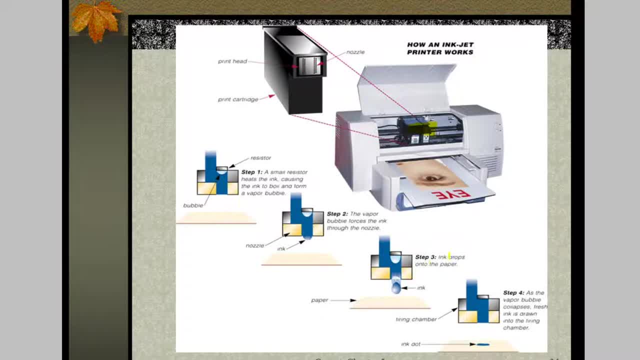 Ink drops onto the paper. Ink drops on the paper, As you can see here In the same way in step 4, As the vapor bubble Collapses, fresh ink And draws into the ink chamber. Now what happens When that ink is drawn? Then automatically Output is produced. 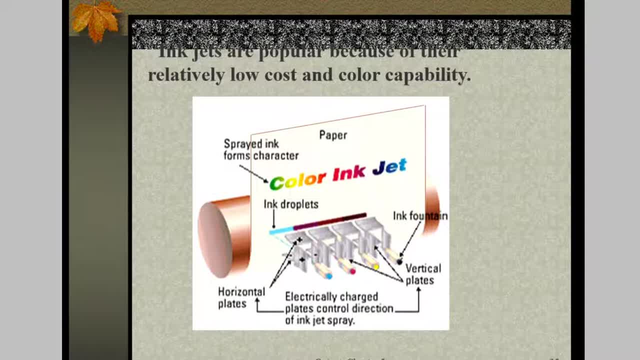 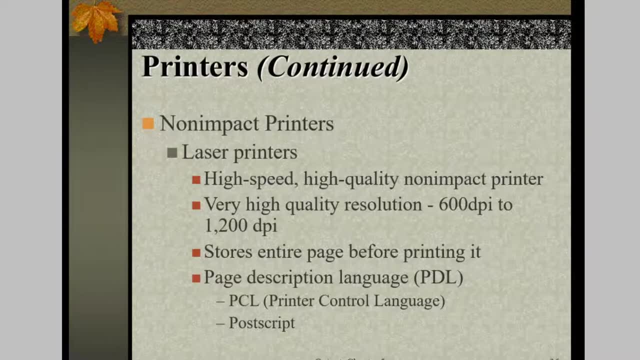 Here we have Color Inkjet Printer. There are pens for different color And we have different color ink, So we get different color output. In the same way, In Non-impact printer, We have laser printers, Which are being used a lot Nowadays, all the printers Which are being used a lot. 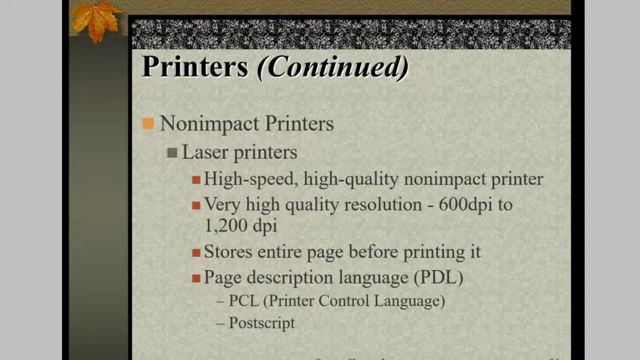 We have the laser printer. We can use laser printer for printing High-speed, high-quality, non-impact printer. Very high-quality resolution, 600 DPI to 1200 DPI. Stores entire page before printing it, As we have all the pages before printing. 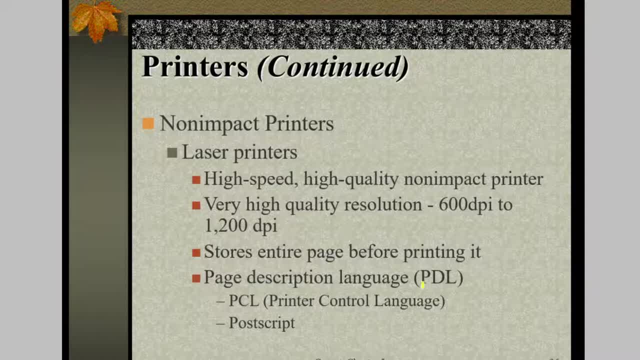 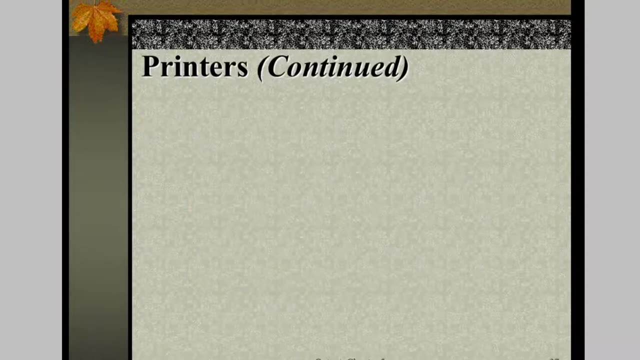 Stores all of them. Page description language: PDL, PCL, Print Control Language. I don't have to tell you all the details. Just keep in mind that laser printer uses laser technology. It is a non-impact printer. Its resolution is 600 DPI to 1200 DPI dot per inch. 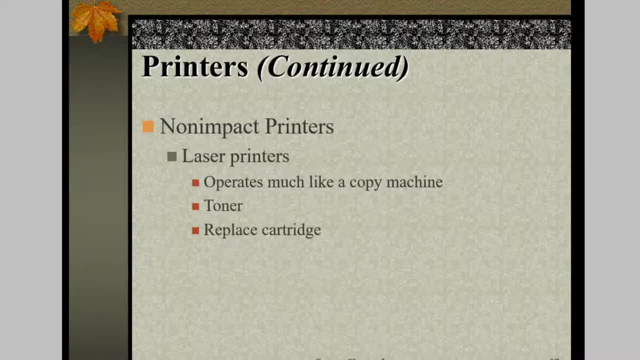 Similarly, laser printer is used for photocopying mechanism. You must have seen photocopier machine. When laser beam is applied on light mechanism, You can see that light is produced, It is copied. It is operated much like a copy machine. 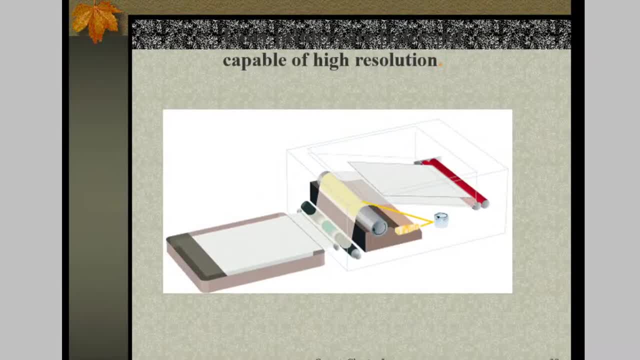 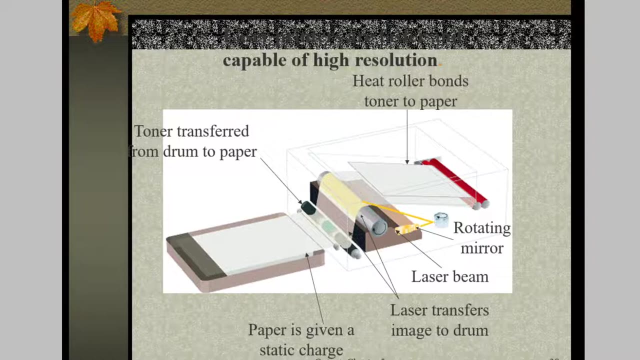 Toner is used to replace the cartridge. We can print high-resolution print in it, As you can see: laser beam, Rotating mirror, Laser transfer. I don't have to tell you all the hardware, But I will tell you that Toner transfer from the drum to paper. 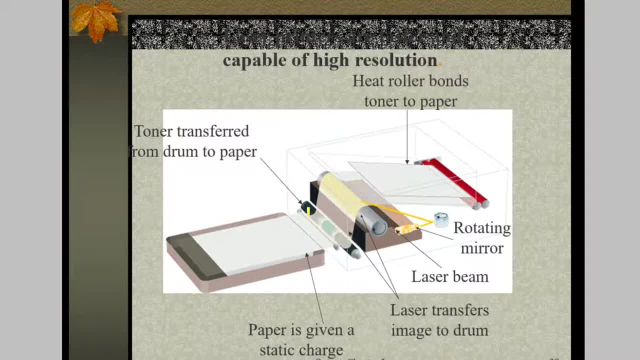 Toner which contains ink, It hits the drum. Charges on the drum One is negative charge And positive charge on the paper. Negative and positive charge are attracted to each other. They are etched on the paper. Paper is given a static charge. 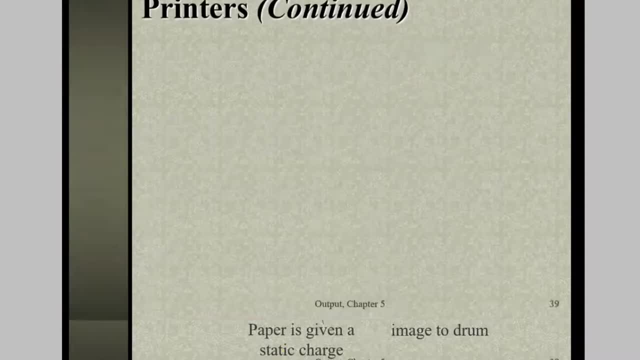 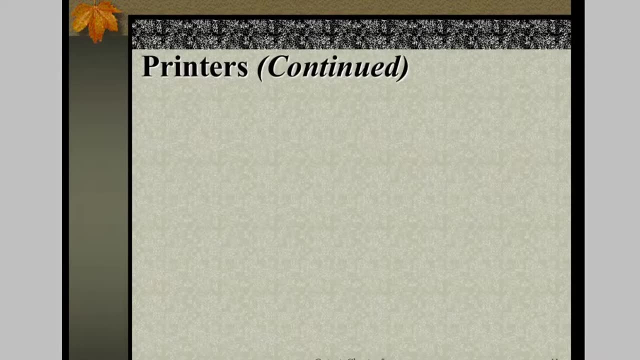 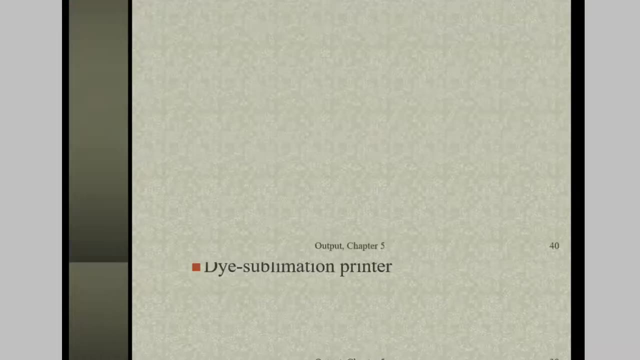 Paper is given a charge, As I told you that there is a charge on it. We have thermal printer like this. We don't need to read these printer types in detail, But you must read it little by little. We have thermal printer. 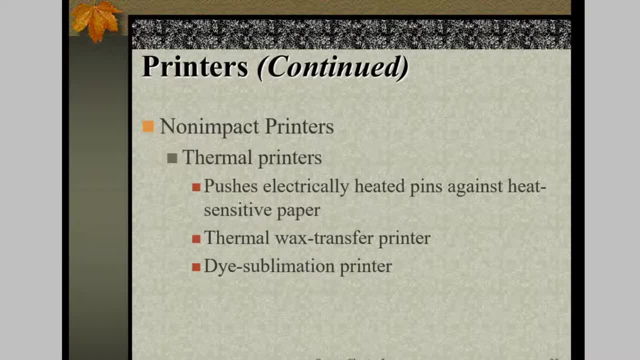 Pushes the electrically heated pins Against heat sensitive paper. Heat sensitive paper- You must have seen photocopy Paper- is heat sensitive If you take heat with it. Take plastic, for example. It is heat sensitive If you take it near the heat. 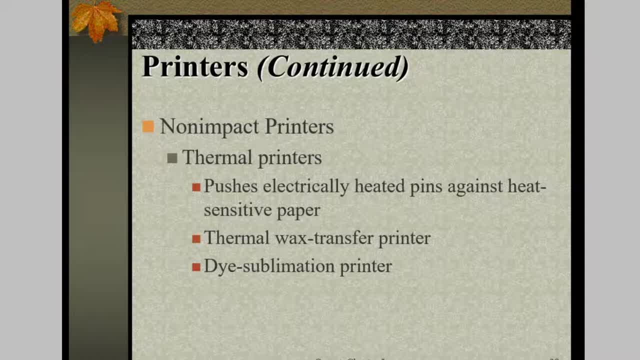 It starts to tear. Similarly, paper is heat sensitive. This is mostly used for your photo, When you make your picture, When you print. This is mostly used for them. Thermal wax transfer printer, Dye sublimation printer, Like here. 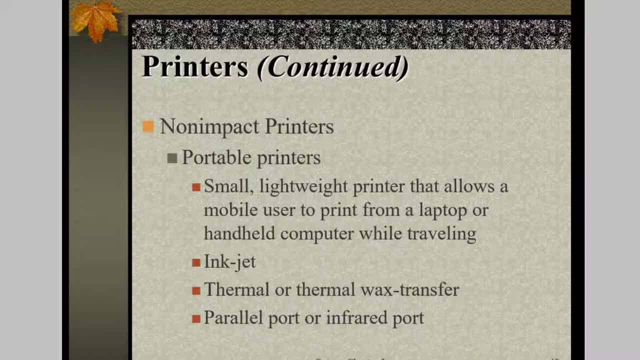 Let me give you an example. These are your pictures, These are photographic. These are heat sensitive paper As soon as the heated pins go with it. According to that, Because of heat sensitive, Our output is produced. Similarly: portable printer- Small lightweight printer. 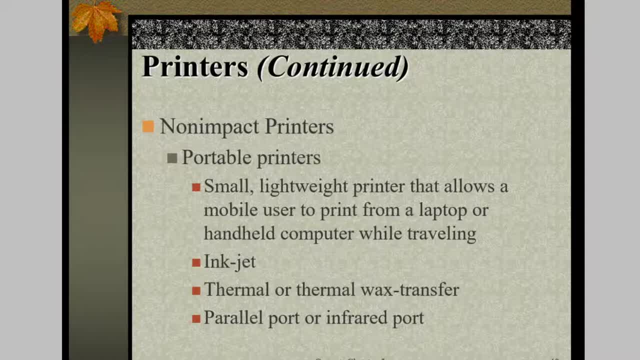 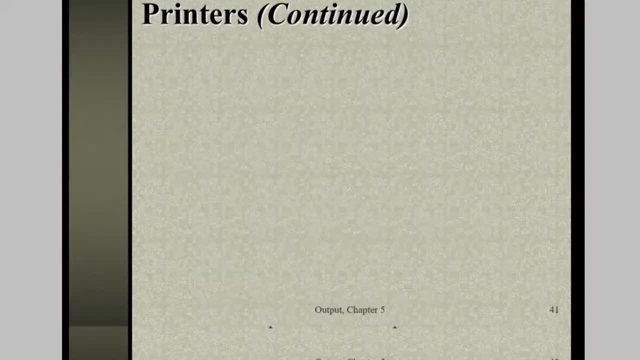 That allow a mobile user to print from Laptop or handheld computer While traveling. inkjet, We have this portable printer. You can easily take it from one place to another. Like we have mobile printers, We have this portable printer. We have small printers. 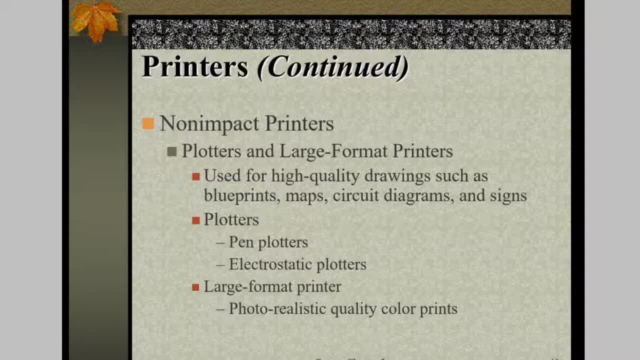 We can attach them to mobile, We can print anywhere. Similarly, my children, If we talk about Plotters, Plotters, We have a printer, Big printer, Through which Graphics are printed, Like you, Penaflex. 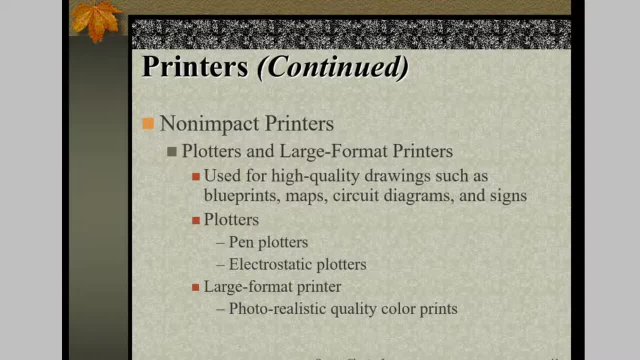 Like these, Through which Plotters are printed. Plotters are large format printers Used for the high quality drawings Such as Blueprint, map, circuit diagrams, Sign, sign print And other things You can print with these. 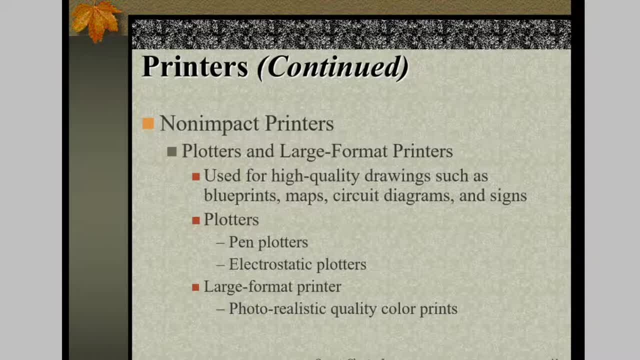 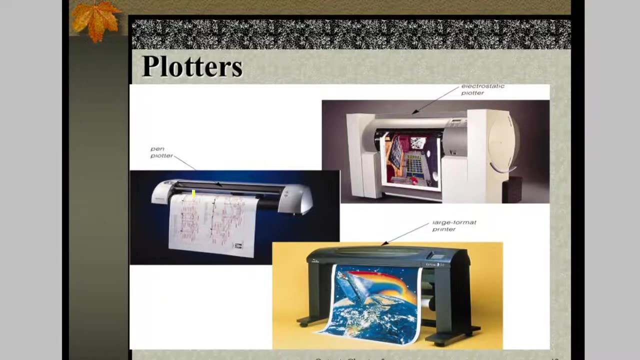 Plotters are large format printers. They are used for the high quality drawings Such as sign boards, pen plotters, electrostatic plotters, large format printer, ink pen, etc. You can see the going back and forth from left to right. 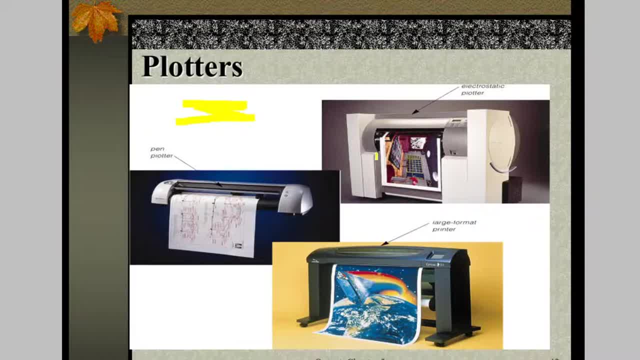 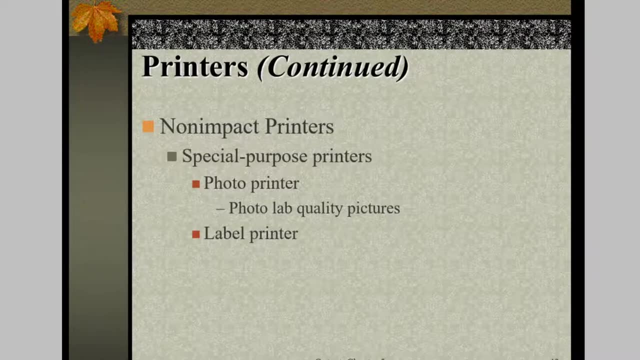 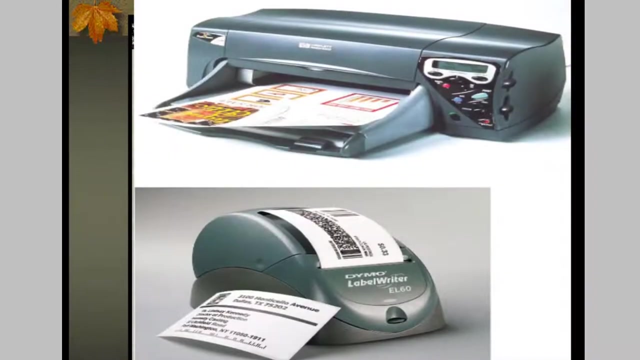 Just like the paper moves its hacia holter vertically, In the same way there is an electrostatic plotter, which is a large format printer in which we have big plotters in which we print graphics and Panaflex. In non-effect printers, special purpose printers, come photo printers which we use to print photos, photo lab quality pictures, label printers, as you can see here. 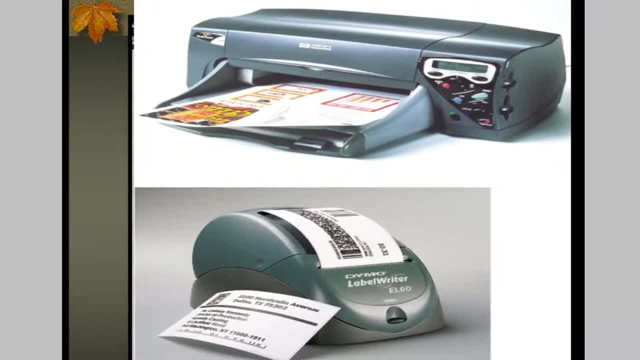 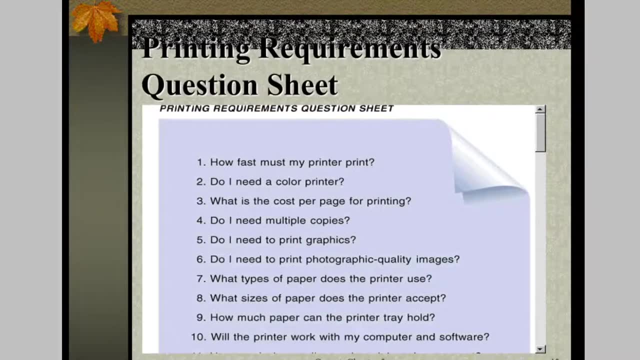 What is special in it? It is used to print our photos or, as you can see here, to print tickets, etc. Similarly, the printing requirement question sheet. what do you have to do? How fast is my printer? How fast is my printer? Do I need a color printer? 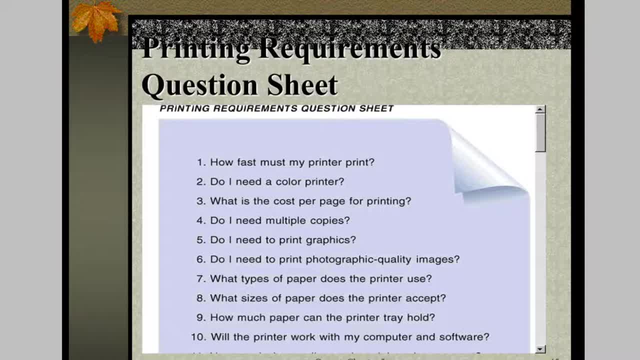 When you go to buy a printer, you have to keep these things in mind. What is the cost of per page? How much is the cost of one page? Do I need multi-copies, Multiple copies? Do I need single-side? Do I need double-side? Do I need to print graphics? 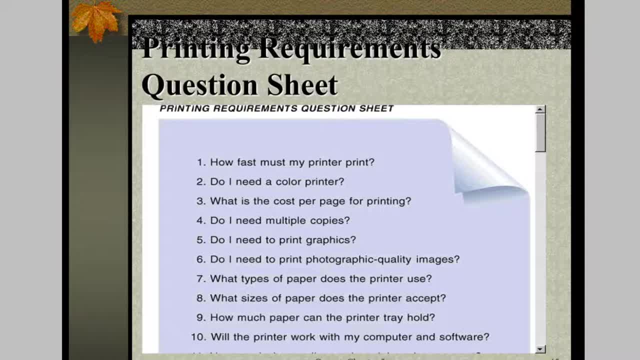 You have to read out all these things and see what is our printing requirement question sheet. When you go to buy a printer, you have to verify all these things first. If you have to purchase a printer, you will tell them the requirements that we need. 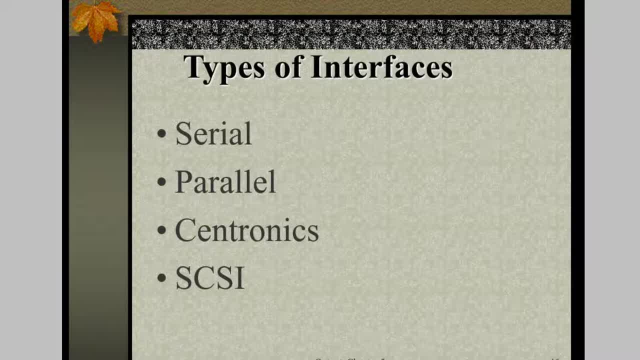 The types of interfaces are serial parallel centronics, SCA Scalpel. The types of interfaces are serial parallel Scalpel. The types of interfaces are serial Scalpel Of the oscillators. we have AA, MRI, we have SCL, etc. 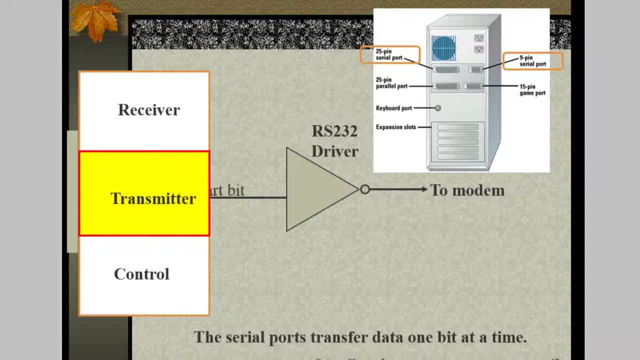 Of the oscillators. we have SCAs, metham அB and we have the serial port transfer data one bit at a time, which is like data being transferred from one port to another. Alright, now the serial port transfer data one bit at a time. 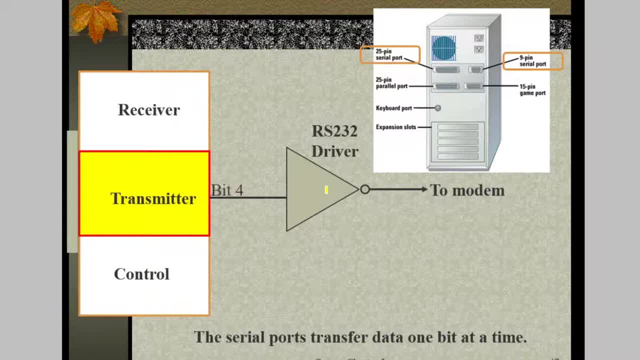 These are the serial ports which we have in the sector of our devices, As I told you last time that we have a serial port and a parallel port, So we can see that the transmitter is connected to the serial port of the device. 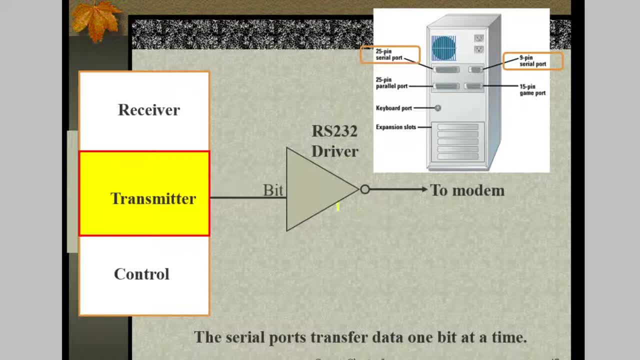 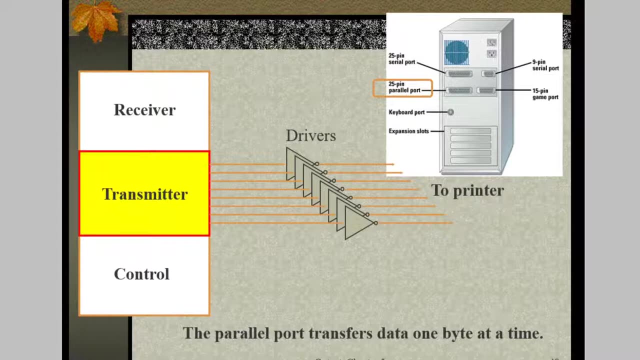 When it is connected to the serial port of the modem, the data will be transferred one bit at a time. Similarly, the serial data transmission is relatively slow. Why? Because the data is being transferred one bit at a time. Similarly, when we talk about the parallel port. 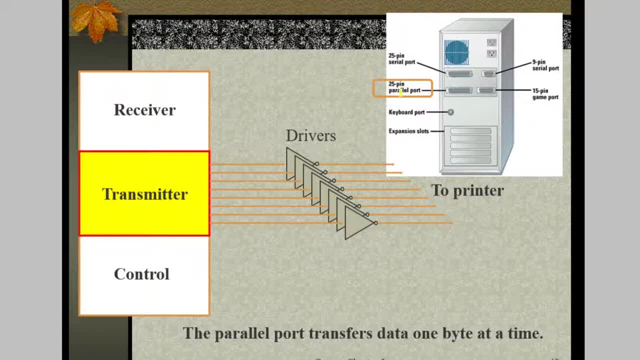 Now you must have an idea that we have 25 pin parallel ports. We have a 25 pin serial port. This is the serial port above. This is a 25 pin parallel port, So we have a 9 pin serial port. 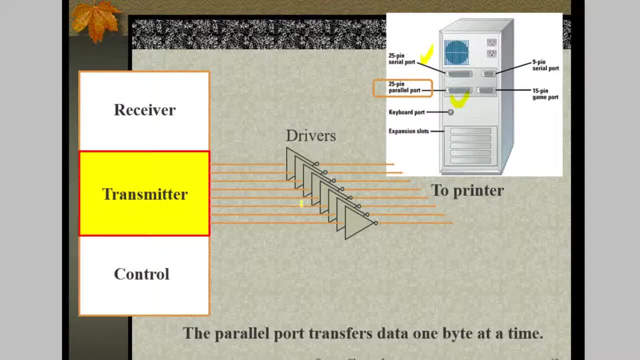 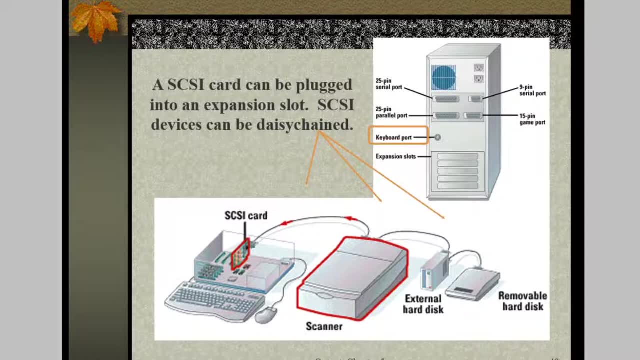 So see how many bits are being transferred at a time. So what will happen to it? It will be fast. Similarly, a SCSI card can be plugged into an expansion slot. We have a serial, As we talked about. SCSI devices can be displayed. 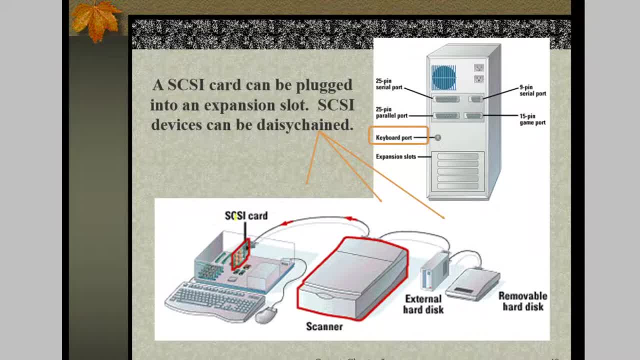 We have SCSI devices. As you can see here. SCSI cards have been installed, Scanner has been installed, External hard disk has been installed, Removable hard disk has been installed, So we have different devices connected to it. How does it work? 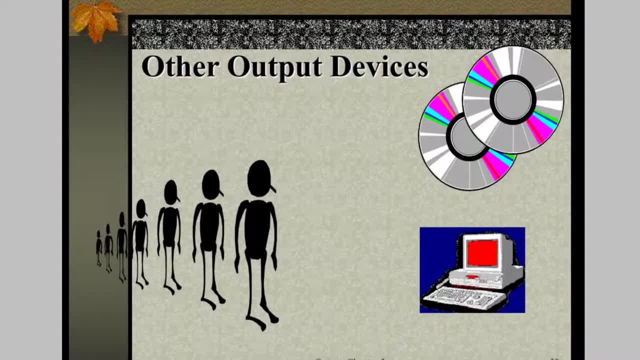 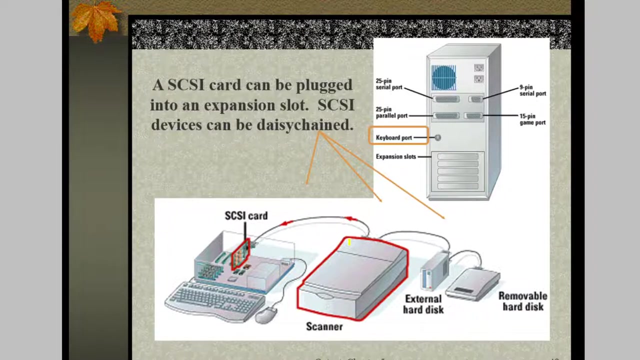 We will see that now. So what do we have here? Output devices? We have other output devices. We have to see that. So in our SCSI we do the setting ourselves. We have these SCSI devices Like we have setting characters. 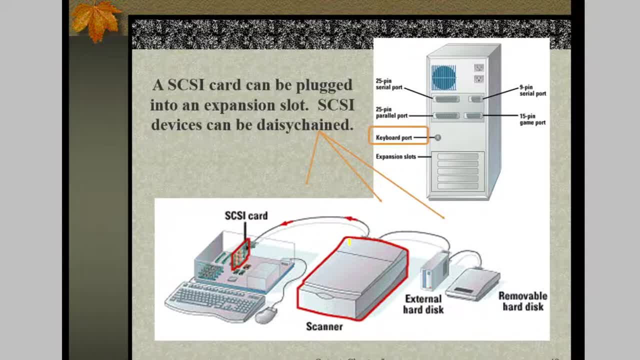 And if we talk about SCSI Action style ideas, All these are present in these devices. As you can see here, SCSI card is installed in our system. It has a scanner like this. With the scanner, what will happen to us? 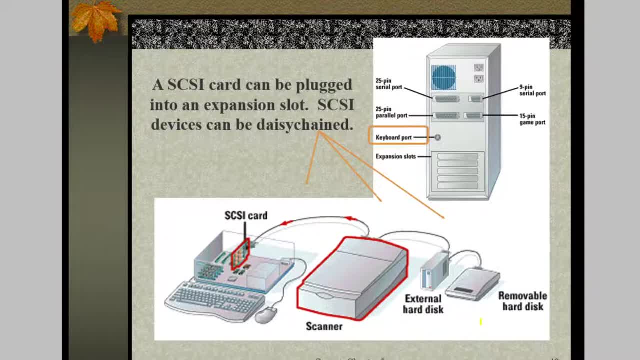 It will be collected. Then external hard disk is there, Okay, And we have to see these things. What are the things we have available? Okay, Then NCID cards are available. Okay. Now, my hope is, AXMS has opened, Okay. 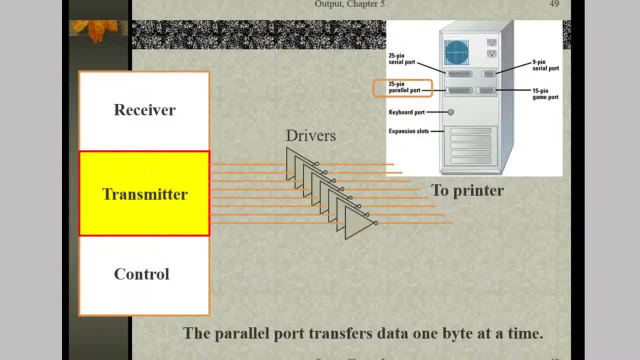 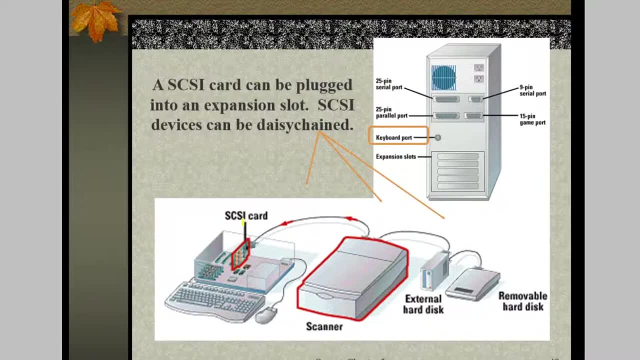 Now, let me wait for. with this, Now, the way that will not open here is few seconds. Now let me wait for a minute. Ummm, Ok, Okay, This is fact. Oh, and cordless connection: Ok, So required. 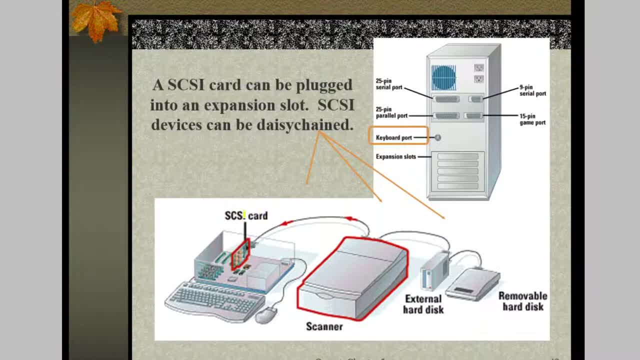 My children. My children- I mean to say that I was a little busy because I could not answer to you Here. all the ports: First we talked here. we talked about serial ports, parallel ports. Now we're talking about SCSI devices. We don't need to go into details of these small devices. 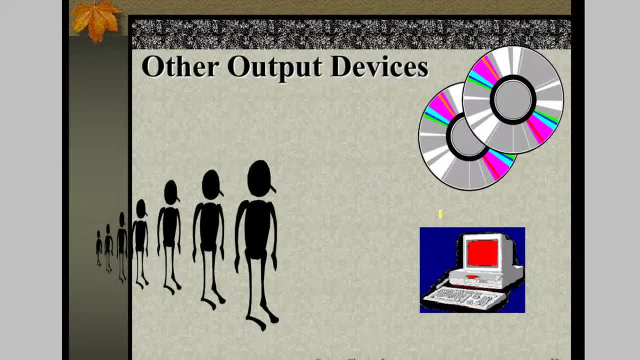 Similarly, if you look at these, we have output devices. I will show you the output that we have. Like these are macro forms. We can also see the output on them. Similarly, CD-ROM audio output, We will have a device. 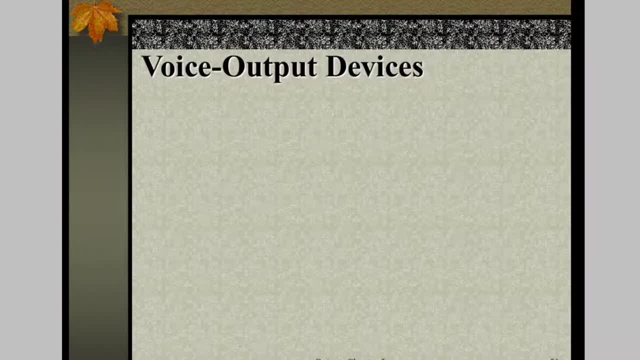 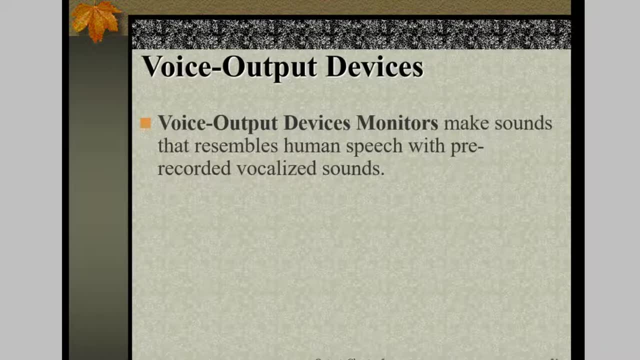 We have robots. All of these come into the output devices. Now we have voice output devices. Voice output devices monitors- make sound that resembles human speech without pre-recorded vocalized sound. I will also tell you about the SCSI devices that we have discussed. 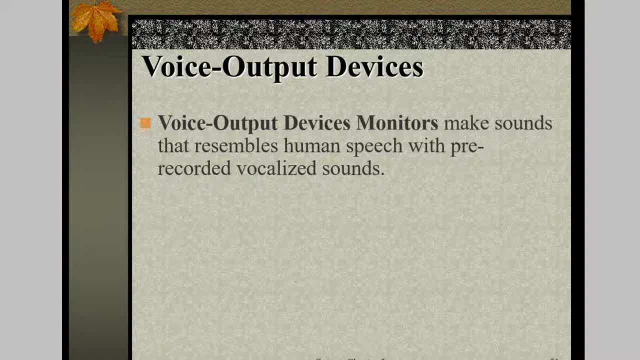 Basically, we have a set of parallel interface standards developed by American National Standard Institute for attaching the printer disk drive. We have external devices to attach them. SCSI devices were developed. These devices were present in our system. We attach other devices to them. 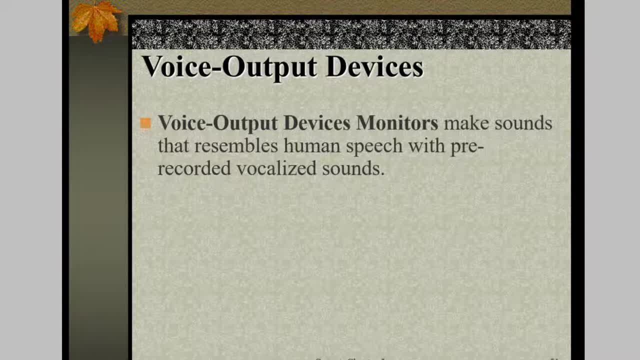 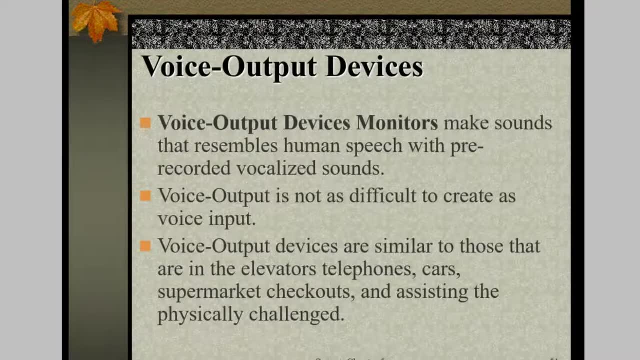 We have voice output devices. We have speakers. Voice output is not as difficult to create as voice input. It is not as difficult to create voice output as we have voice input devices. We have to convert them according to the system. Similarly, voice output devices are similar. 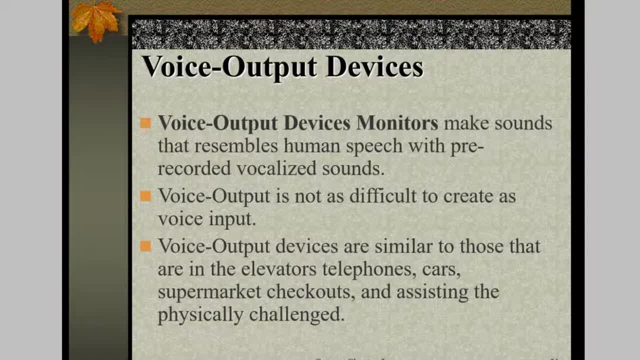 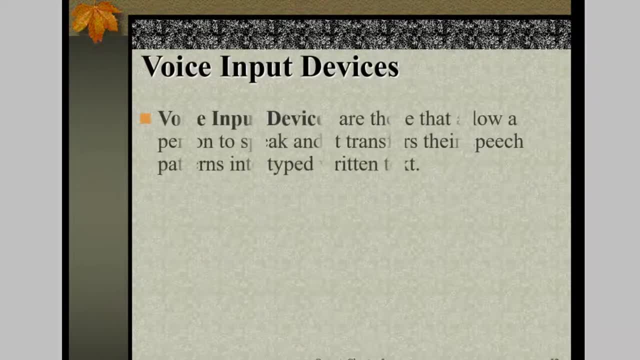 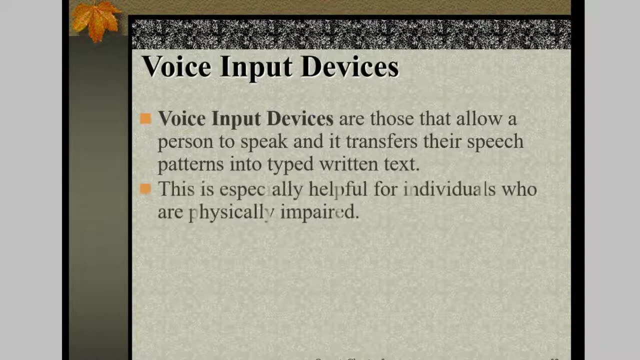 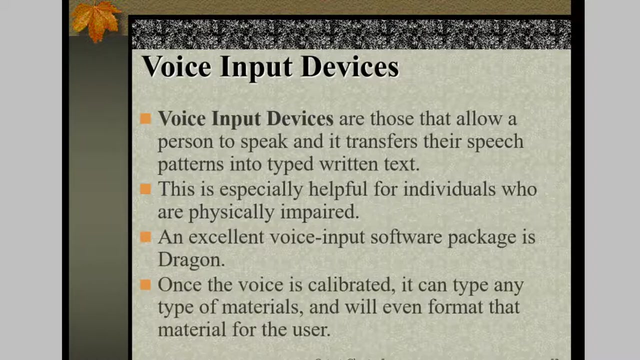 To those that are in elevators, telephones, cars, supermarkets, checkouts and assisting the physically challenged voice. You know that we have voice input devices that take our voice into our system. We call them voice input devices. Similarly, we have already discussed about input devices in detail. 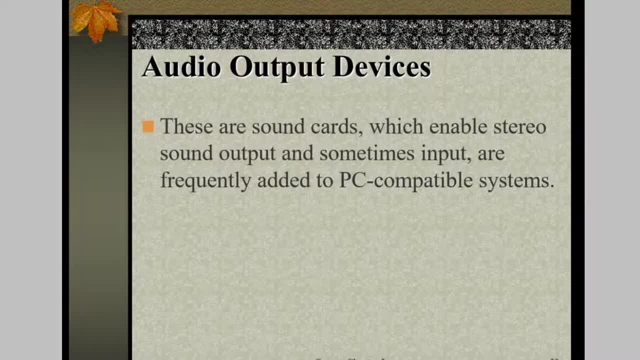 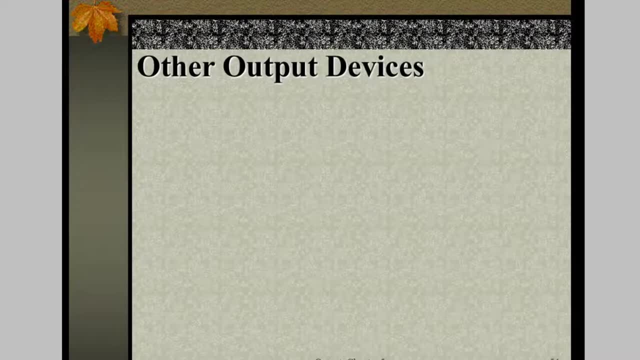 That is why audio output devices are the sound cards which enable the stereo sounds. Audio output and sometimes input are frequently added to the PC-compatible system. Similarly, we have other output devices. We have a fax machine, Because the output is generated on the fax machine. 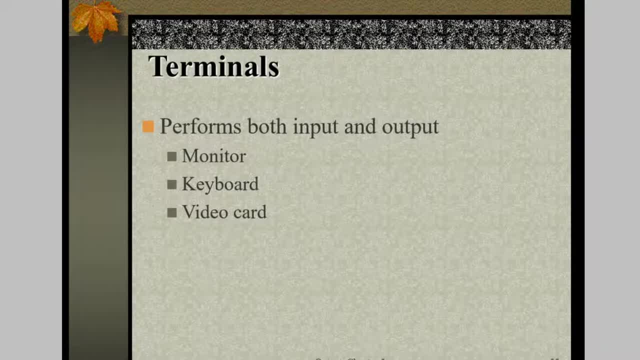 Similarly, we have a terminal Perform both input and output. We have a terminal which has both input and output. For example, we have a monitor, keyboard and video card. We call them terminals. As you can see, we have a keyboard input device and output device. 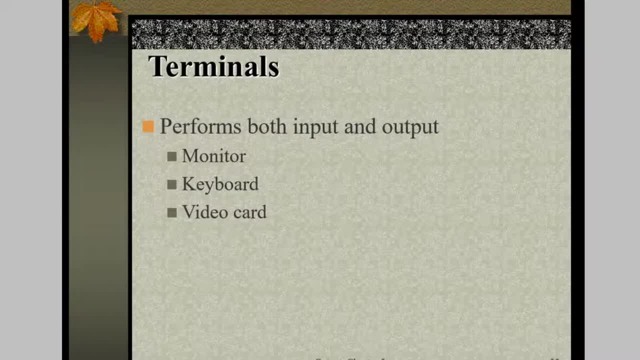 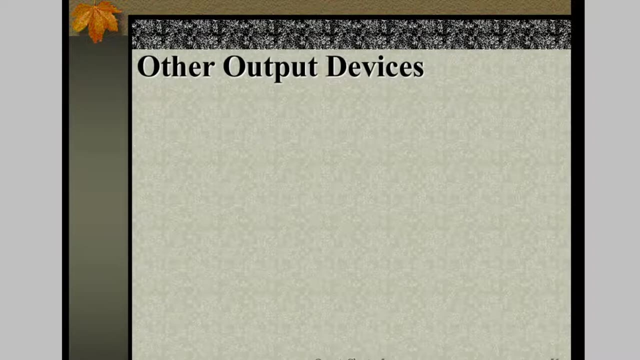 Terminal means that many devices will be attached together. If we have a speaker in our system keyboard, we have an output device. Similarly, we have a video card, We have output devices. If we have a terminal, it means that all the devices are attached together. 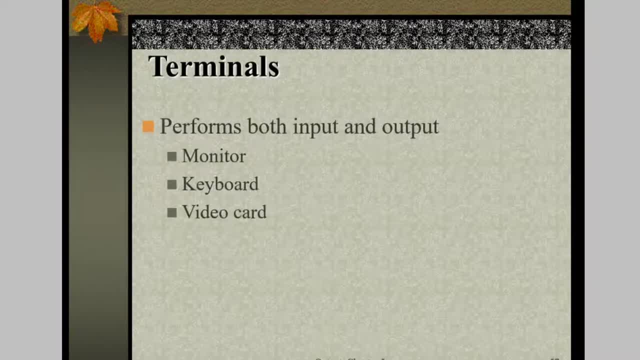 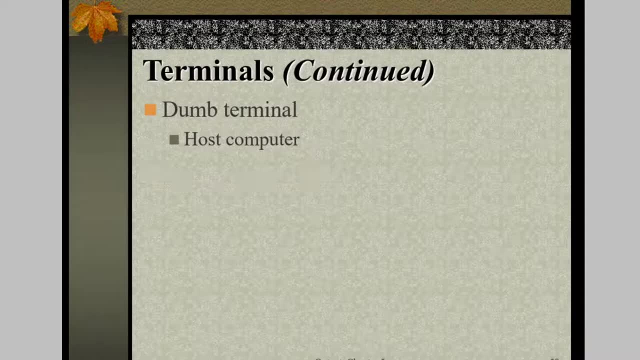 We do not need to tell about the output devices. We do not need to tell about the output devices. We have a terminal. We have discussed that. it performs both input and output. We have a monitor keyboard and a dump terminal. We have a host. 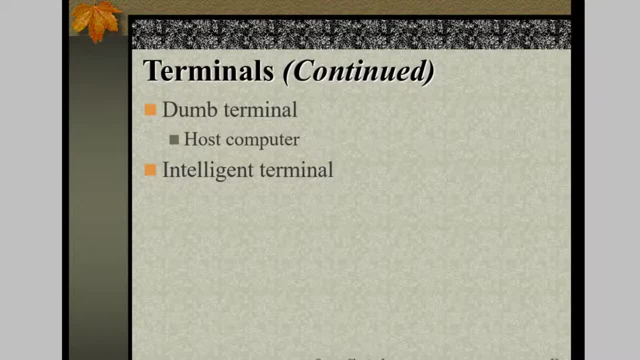 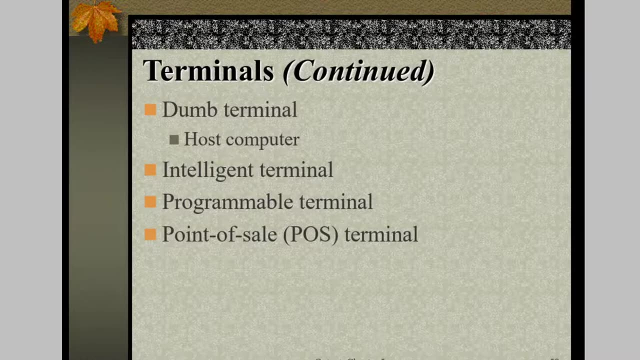 On the dump terminal, we are only looking at the things Nothing else is performing. Then we have an intelligent terminal. Everything is being performed on it, Everything is being calculated. We have a programmable terminal In which we can do programming and coding. 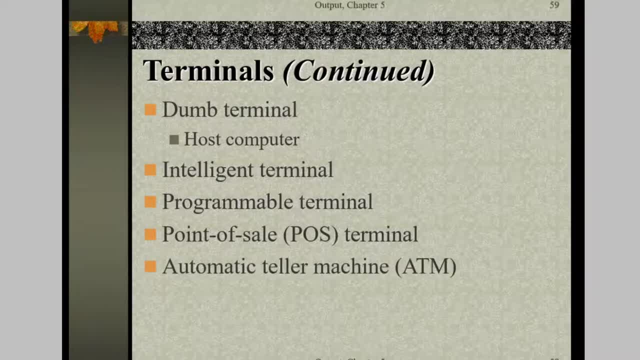 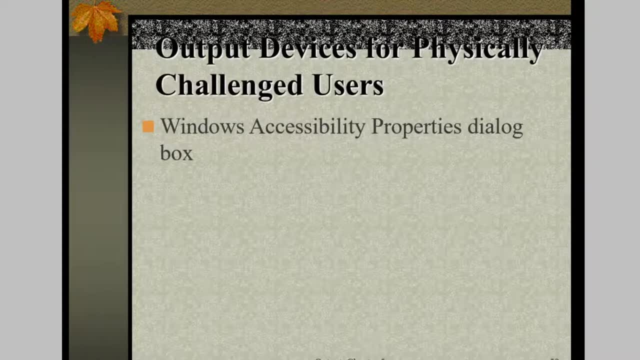 We have a point of sale, We have POS terminals, We have an automatic teller machine, We have an ATM, as you have seen earlier. We have output devices for physically challenged users. We have Windows accessibility properties for users. We have a dialog box. 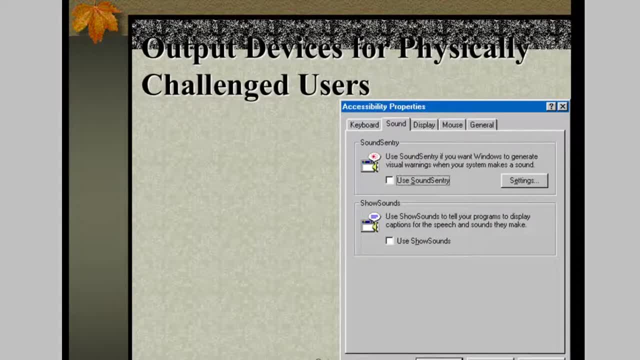 You can go to the dialog box and set it. As you can see here, we have a control panel in the output device dialog box. We have an example of our hardware. We now go to a card that is used for enable and disable that. 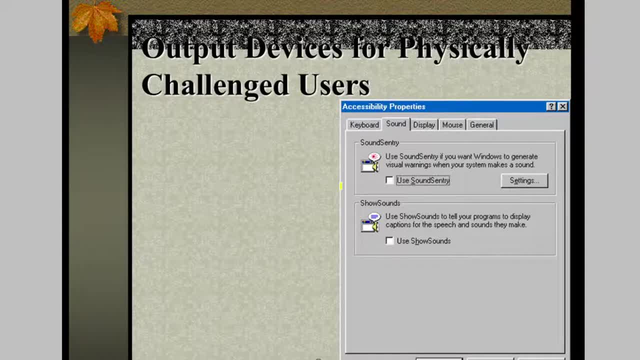 So this setting we have one day You see the lecture of this setting, How we can set its properties together, Like here: you have the keyboard setting. Use sound sentry as to which setting you can do it. Alright, Show sound means at the click. 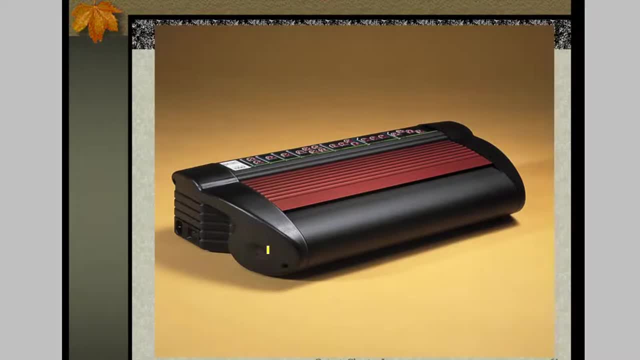 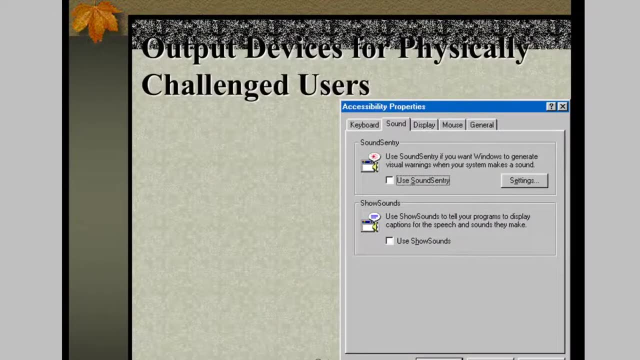 There should be sound coming or not. You can set all things by go through this setting. So what do we have here? Lecture of the output devices. We have different onto use devices. Let us now know about this, how this will work. Output devices. 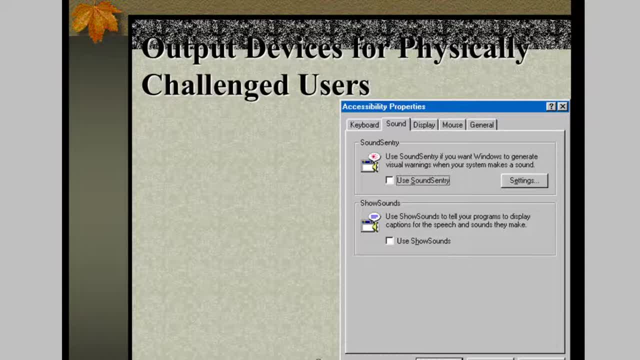 Wish you all best for your upcoming lecture, Which is our technical Basic. things are almost finished. Now we will move towards technical things. In our next lecture We will study storage units And after that We will start our practical. Stay happy. Don't forget to give feedback If my kids have any problem. 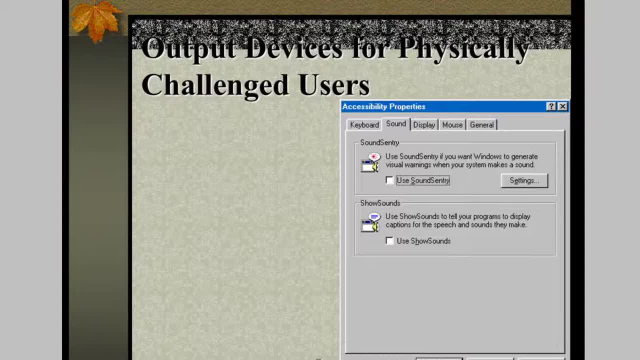 Any question in mind. Write up your question. I am always available for your Answering. I am always available for your Question answering. I have already told you That if 2-3 people Want to come to campus, I will be available on Monday and Tuesday. If you have any issue. 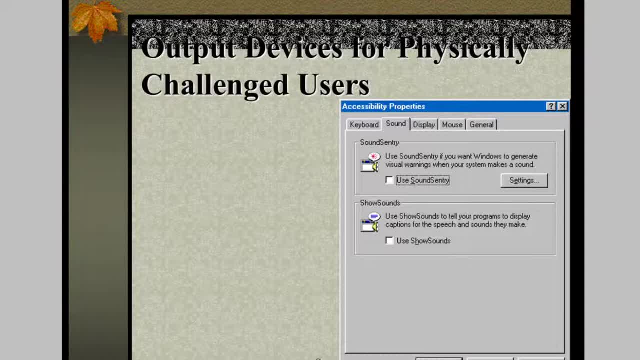 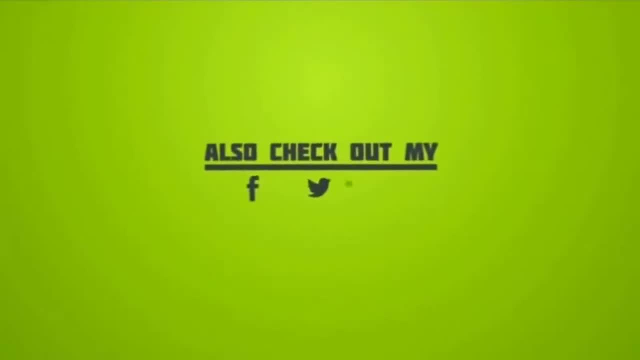 I will guide you. Allah Hafiz, Thank you.